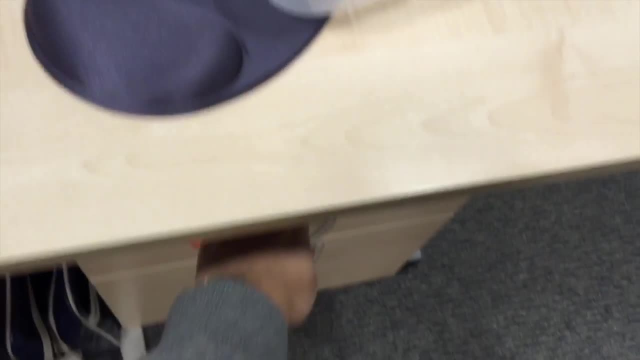 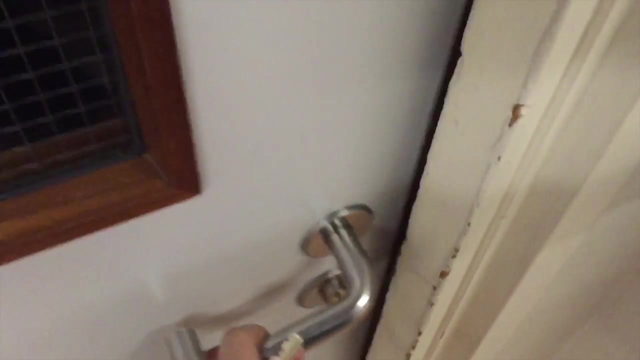 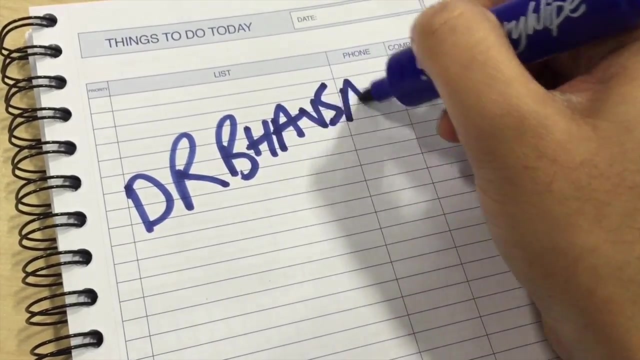 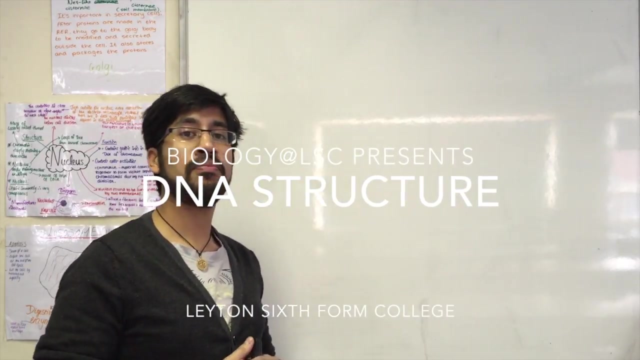 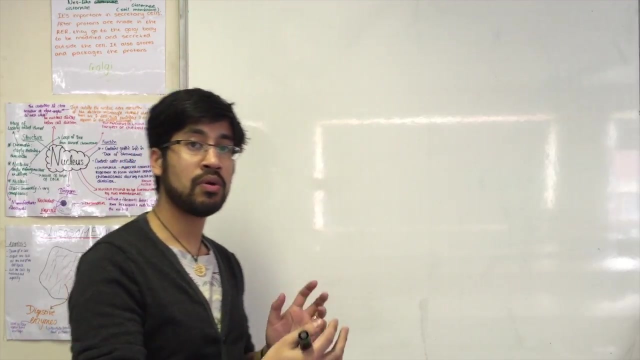 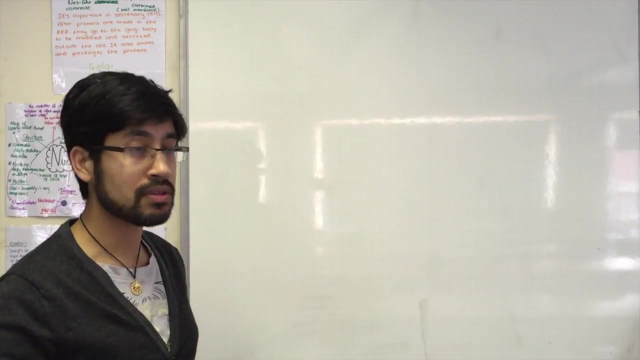 Hello guys. so in this video we're going to talk about nucleic acids, going to go from structure to function. We're going to talk about DNA and RNA and how their function ultimately is to store information and then use that information to produce proteins. Okay, so let's begin. 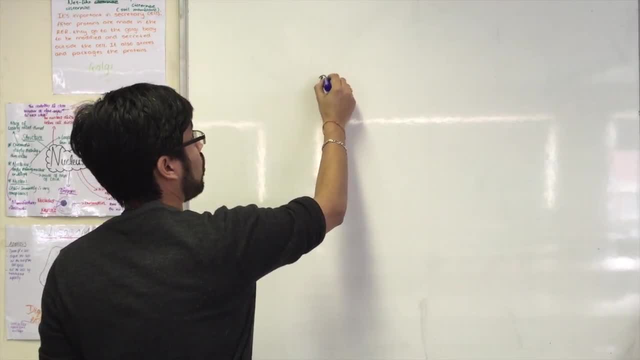 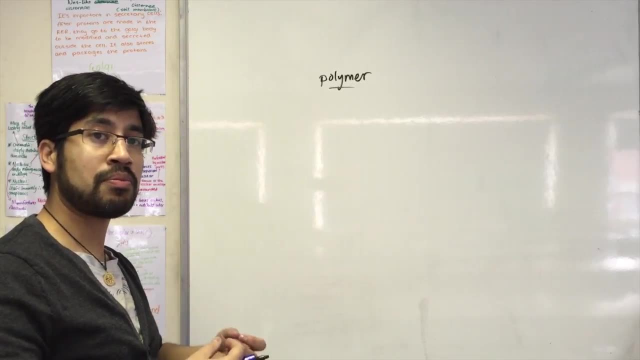 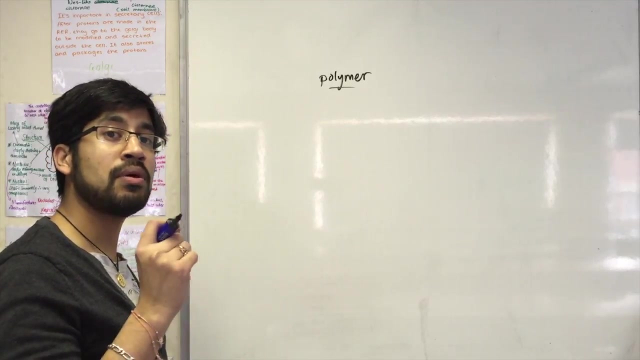 The nucleic acid is a polymer. Okay, so, just like the protein is a polymer and it's made up of the monomer, which is amino acids, we've got polysaccharides, which are the polymer, and they're made up of the monomer, that is monosaccharides. 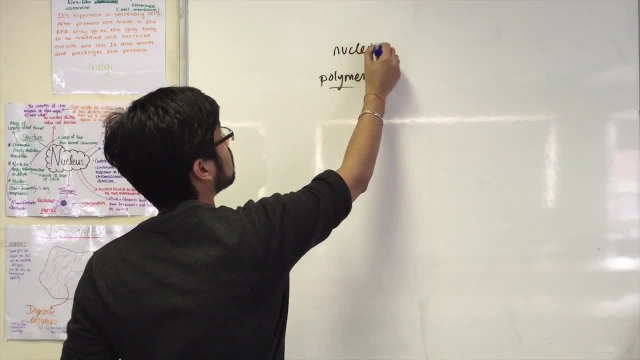 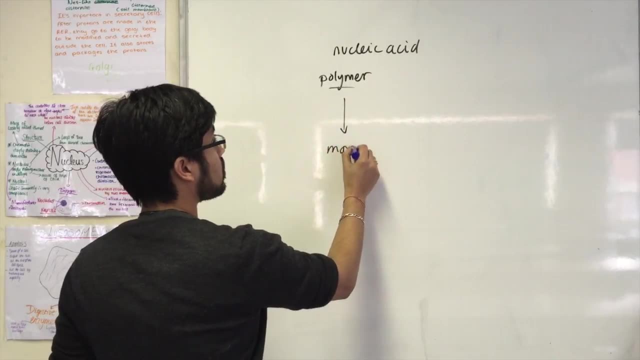 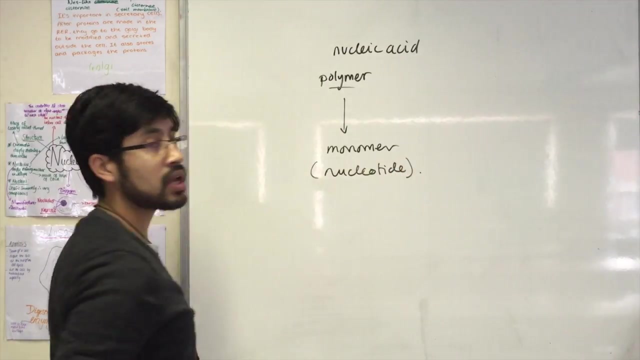 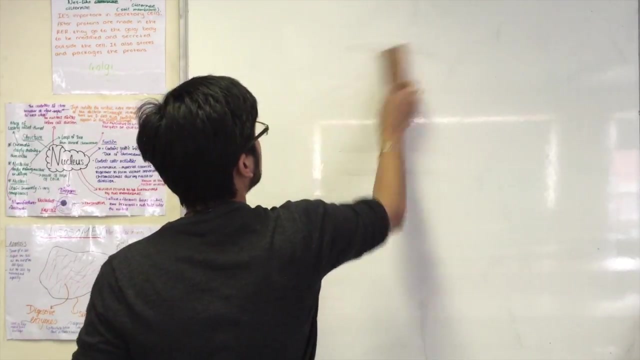 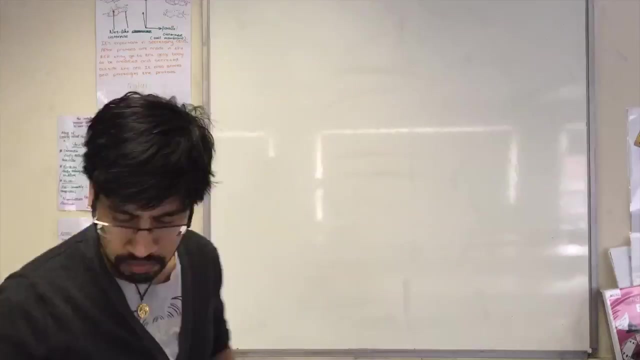 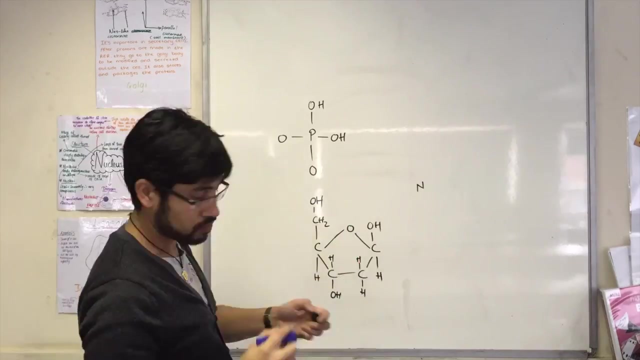 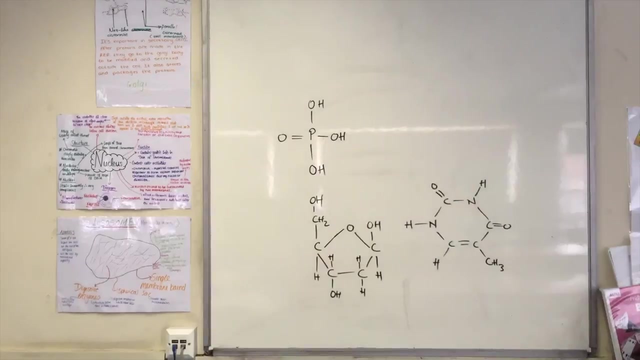 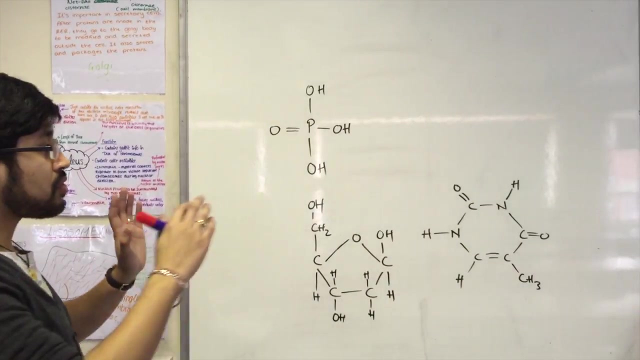 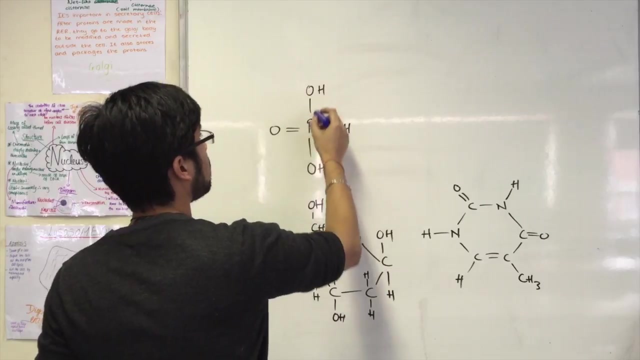 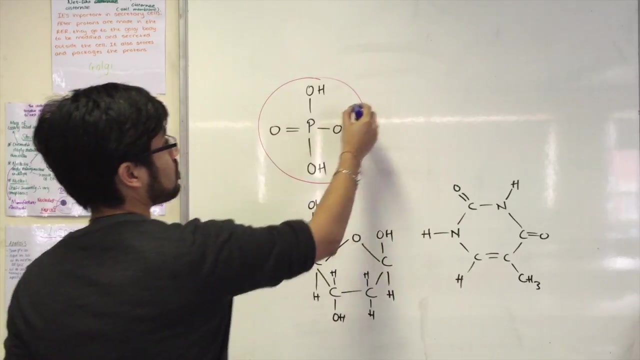 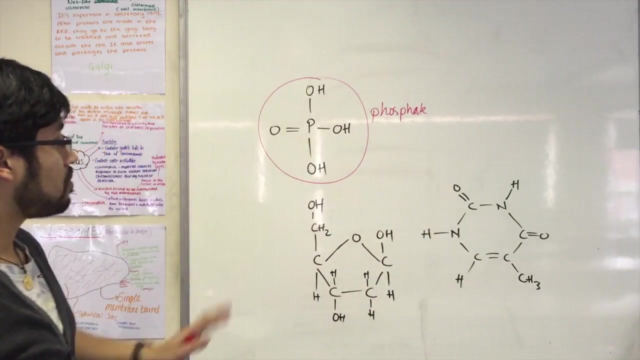 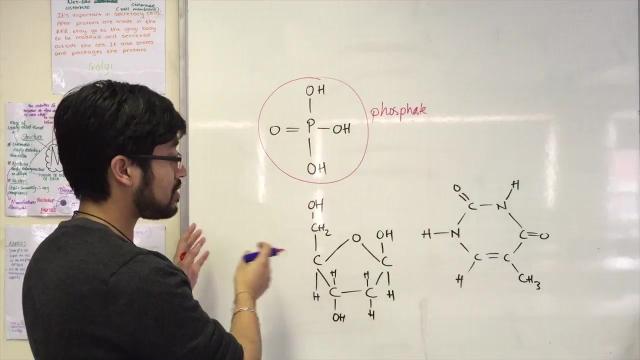 The nucleic acid is a polymer and its monomer is the nucleotide. Okay, so, let's have a look at the structure of that. Okay so, let's have a look at the structure of that. Okay, so, let's have a look at the structure of that. 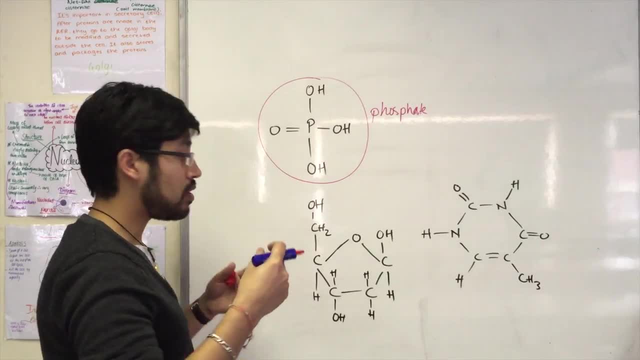 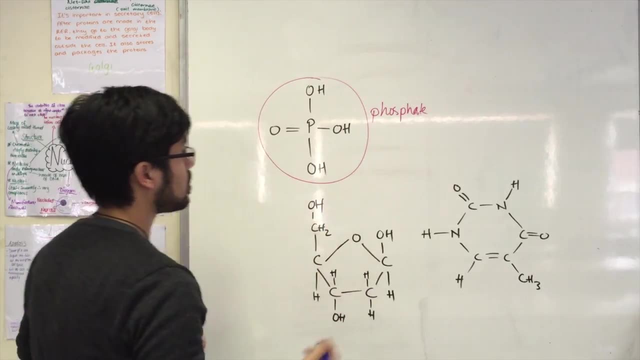 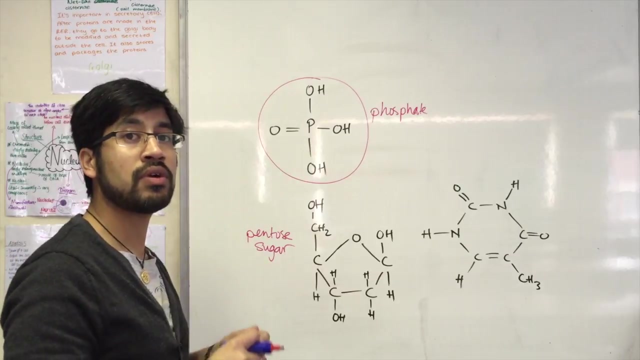 Now, in RNA, this pentose sugar would be different – it would be ribose. Okay, Right, So this is our pentose sugar. So this is our pentose sugar, and here we have one of five different potential bases, or nitrogenous bases. 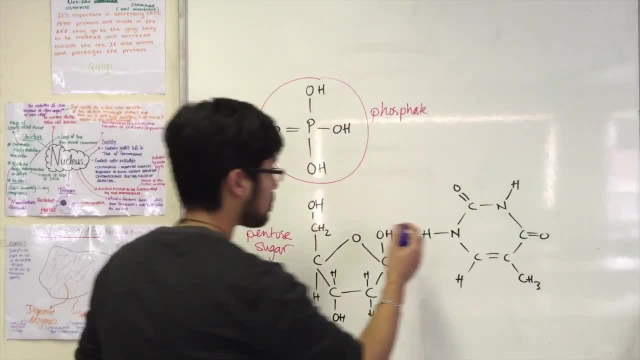 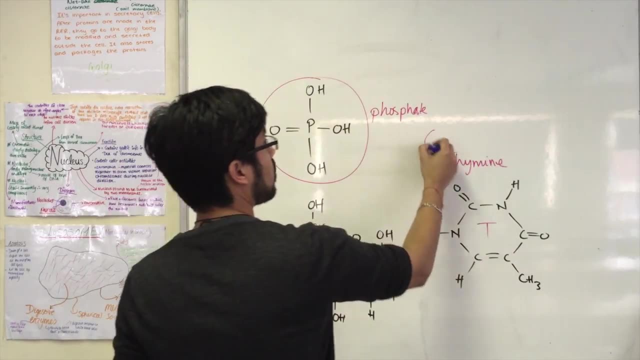 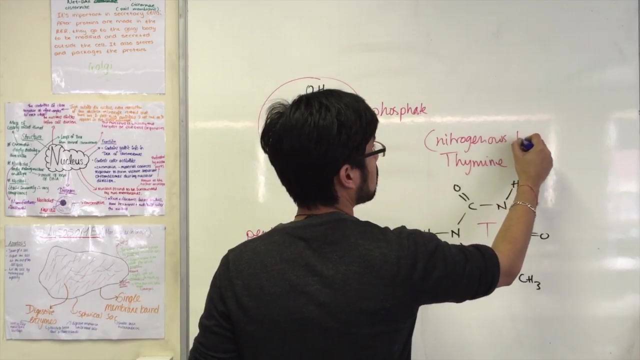 And here we have one of five different possible bases, or nitrogenous bases in this case. case I have here thymine. Thymine is the example that I've got here, but you know, in a general nucleotide we would call it a nitrogenous base. 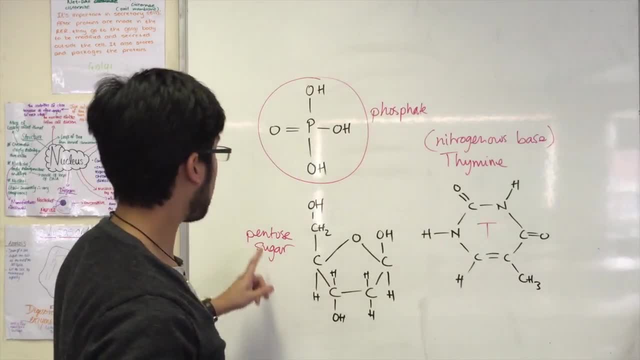 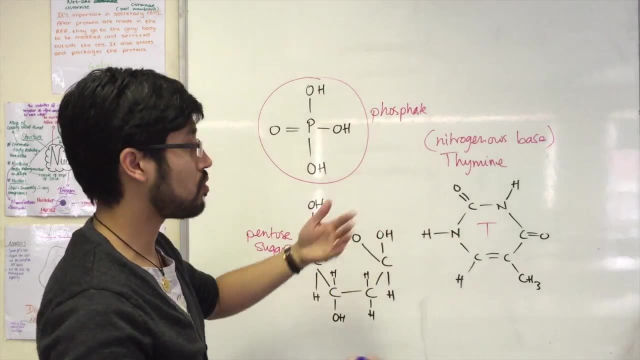 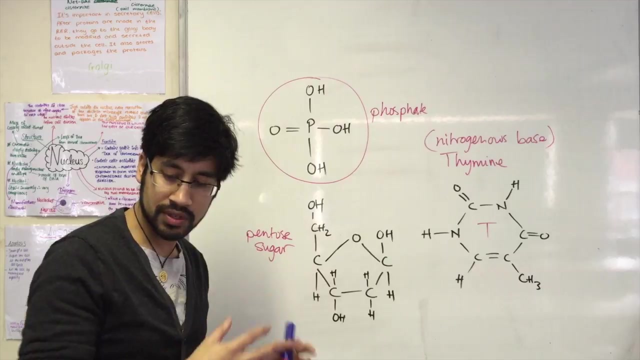 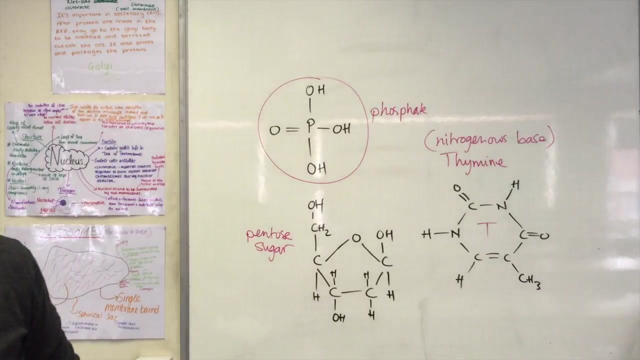 So three components of a nucleotide: pentose sugar, a phosphate molecule and a nitrogenous base. In this case I've got thymine. it could be one of four others. We'll discuss the specifics of bases and their combinations later. So how do these come together to form the nucleotide? 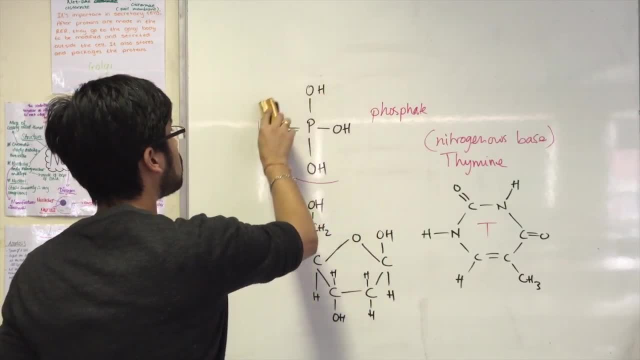 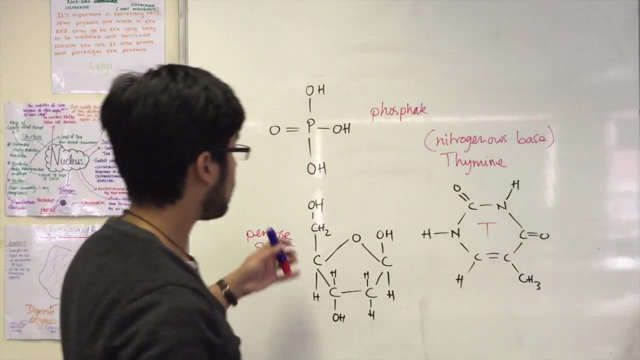 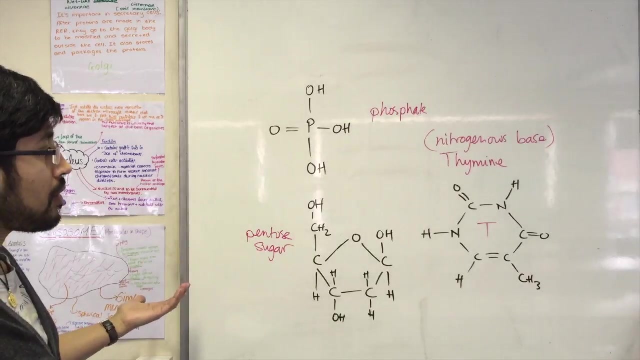 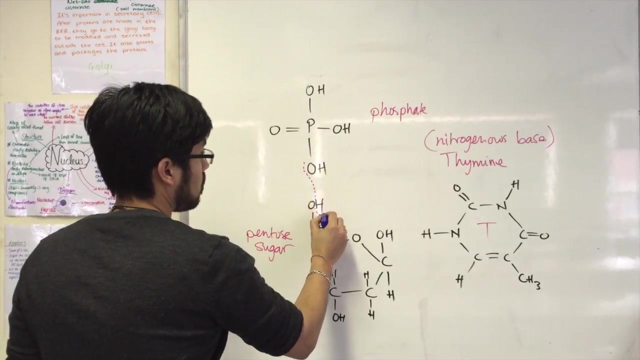 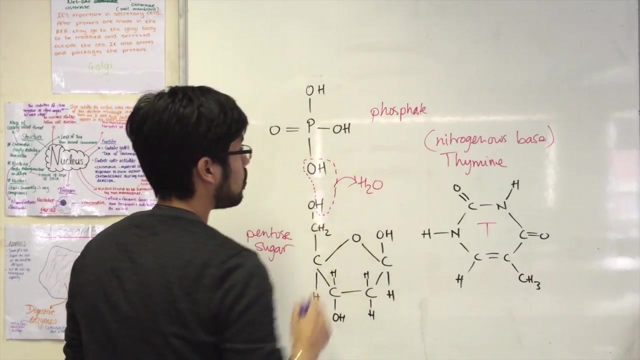 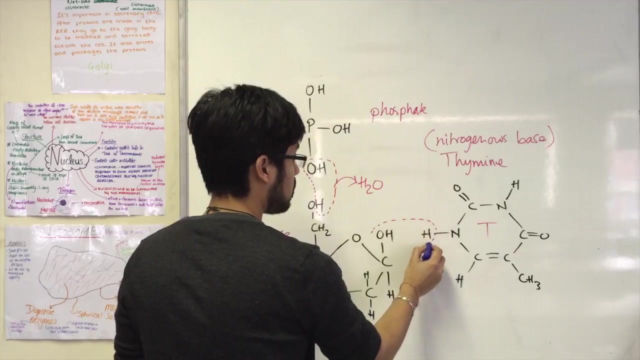 Luckily it's nothing new here. it's our old friend, the condensation reaction. So just looking at this diagram you'll be able to see how it's going to be connected through condensation reaction. Very simply, two hydrogens and oxygen there that's going to form a water molecule, And similarly over here two hydrogens. 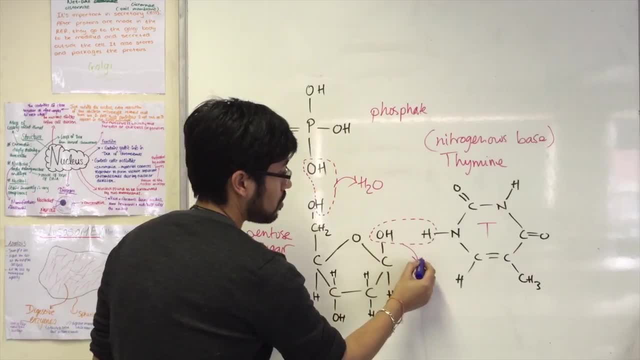 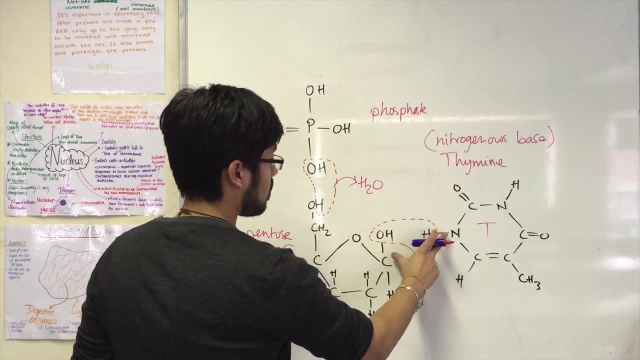 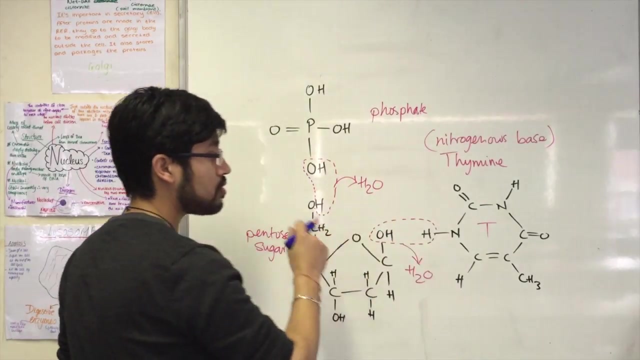 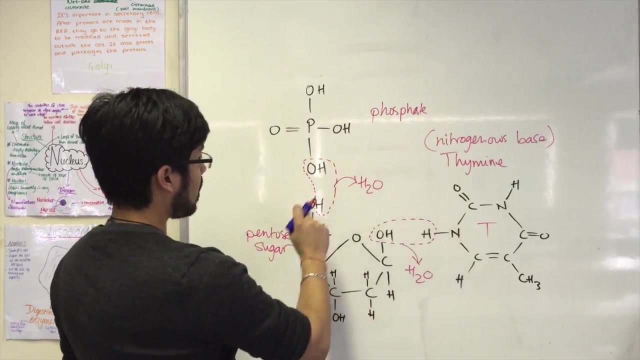 and an oxygen there, and that is also going to form a water molecule. When that happens, the remaining atoms, you know, which all, have lost one bond. they will satisfy their need for a covalent bond by bonding to each other. So in this case, the carbon to the nitrogen and in this case, the oxygen to the phosphorus. 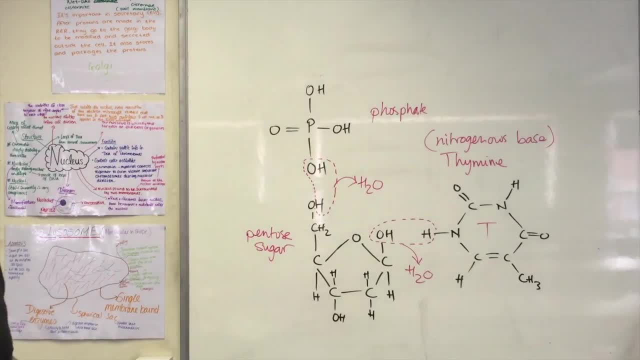 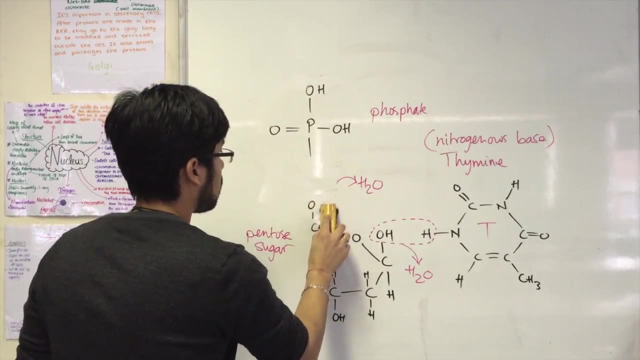 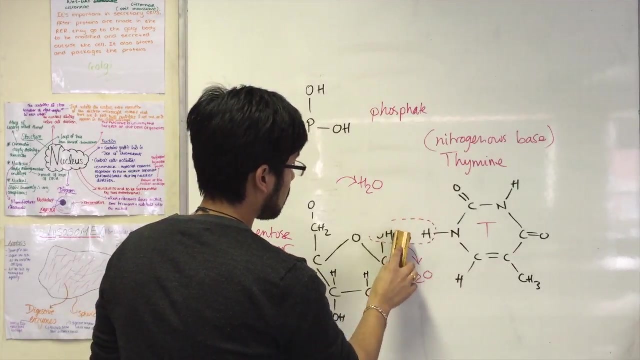 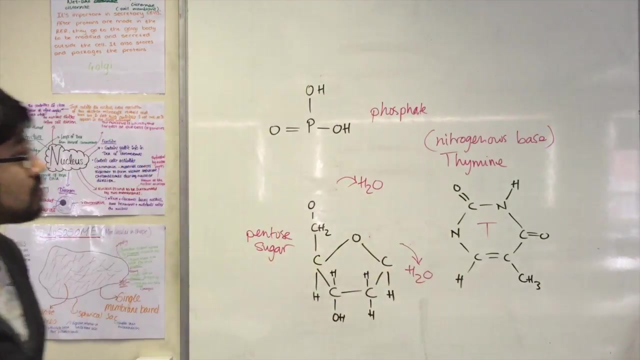 atom. Okay, Right, so let's just have a look at what that would look like. So we've lost the OH there and the H from that O that's not there anymore, And we've lost all of that because that has now become the water molecule there. 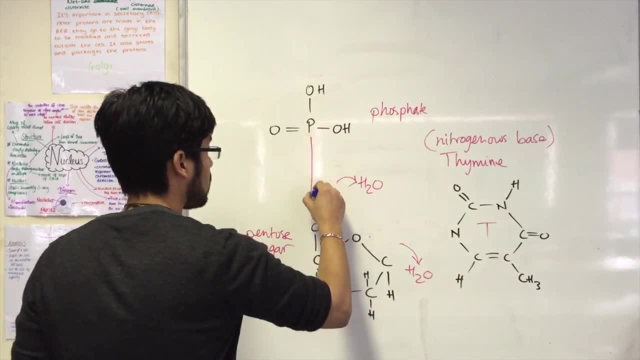 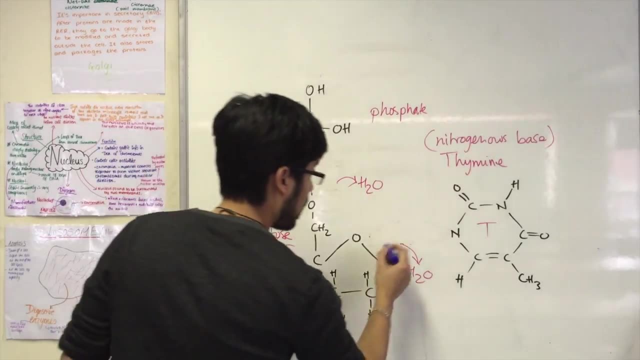 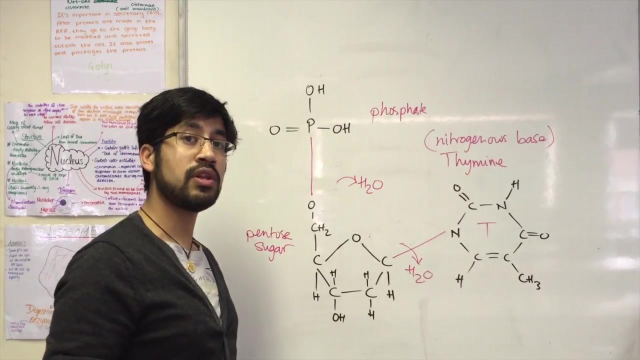 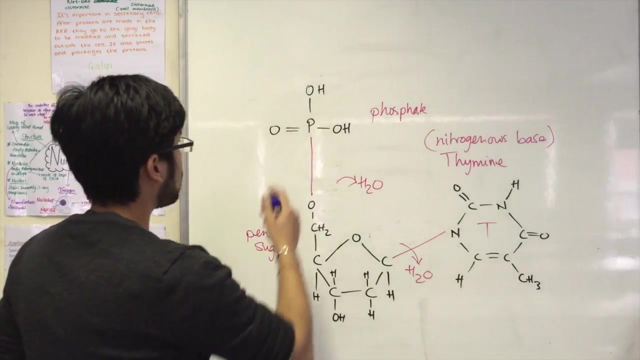 So the new bond which is formed. It's there, Bond lengths not to scale, And there from the carbon to the nitrogen, And thus we have a nucleotide. Okay, so let's just quickly talk about the new bonds that are formed. 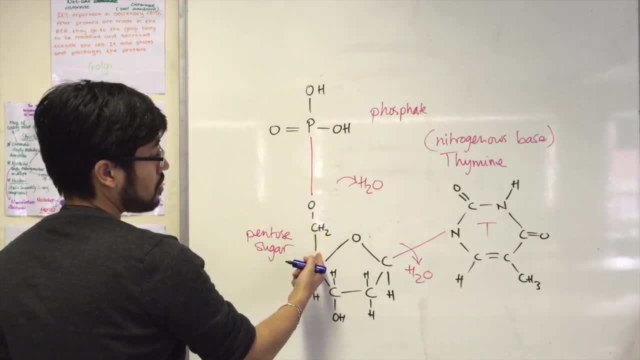 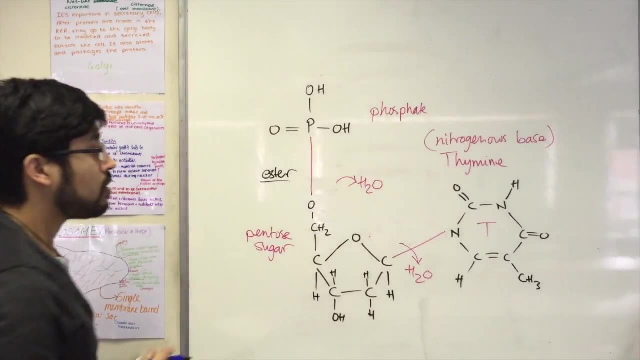 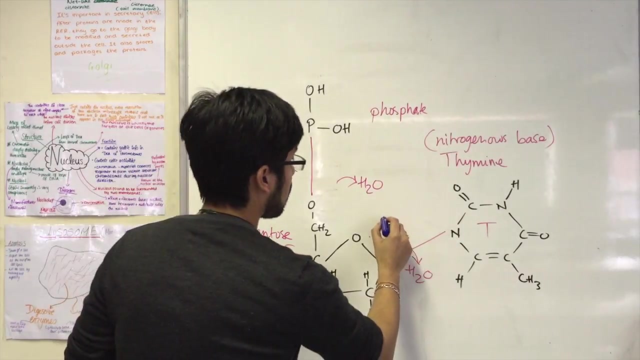 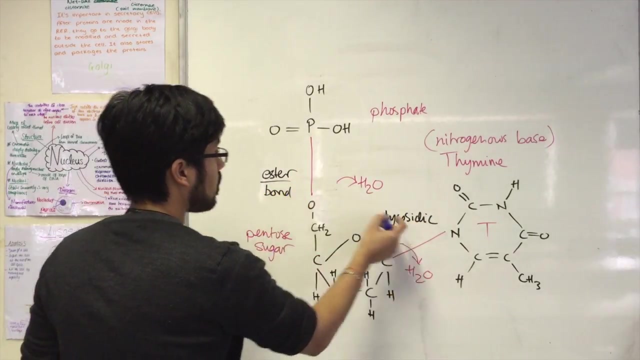 Here the bond between the phosphate and the sugar is called an ester bond- Okay, And the bond between a glucose and another group is called a glycosidic- Okay. so here we have an ester bond and here we have a glycosidic bond. 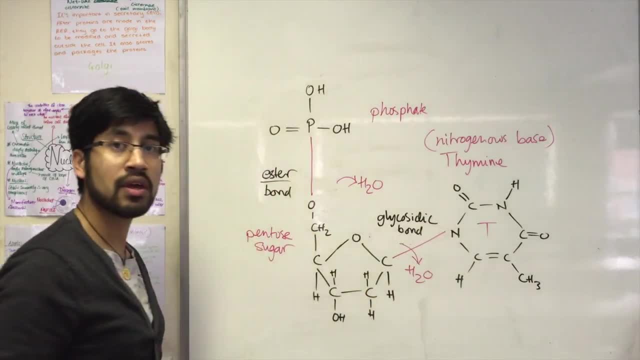 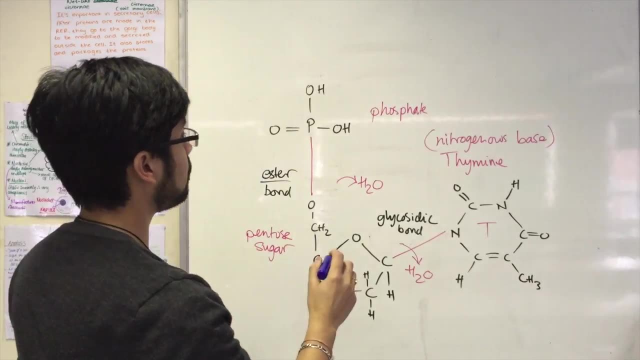 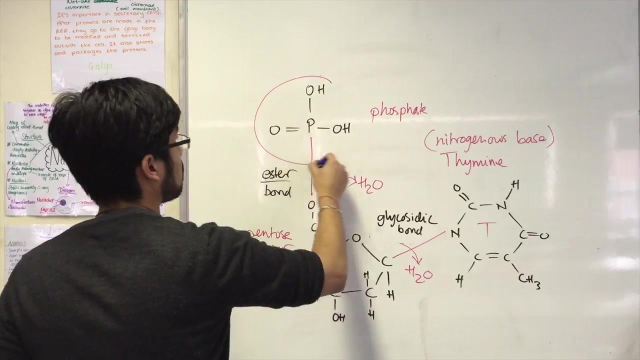 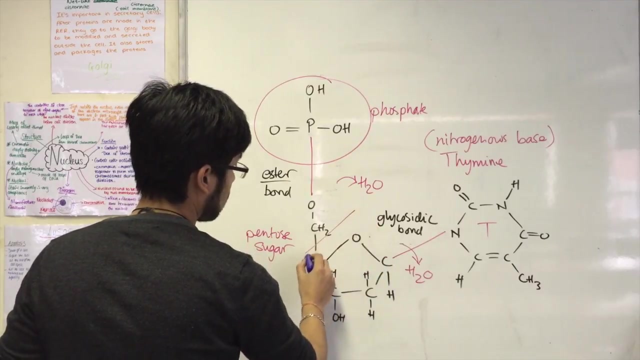 Okay, And thus we have the three components of our nucleotide In all the following discussion I'm going to simplify this right down to a much simpler organization. Just to keep us sane, I'll denote the phosphate group with a circle. I'll have a kind of pentagonal shape for the pentos. 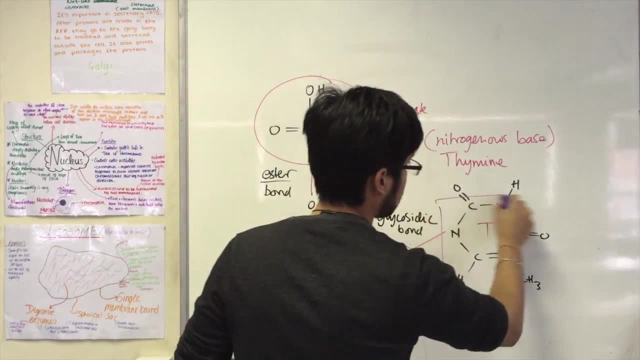 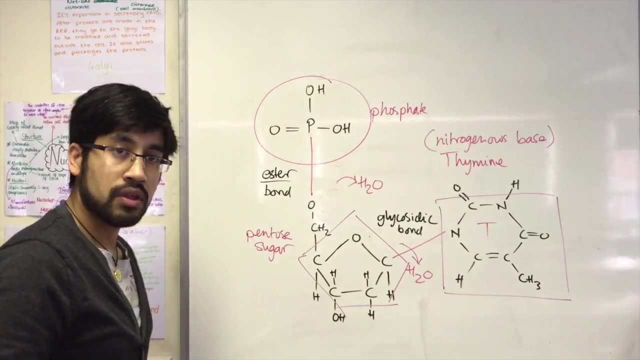 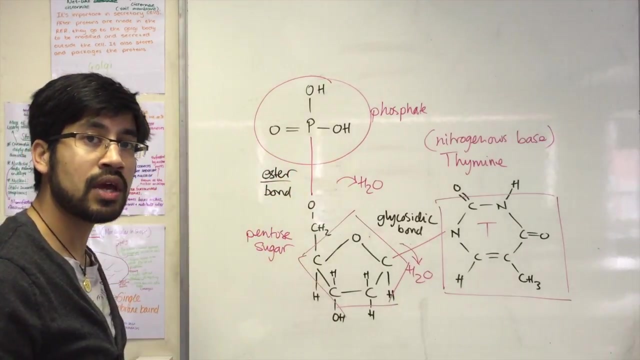 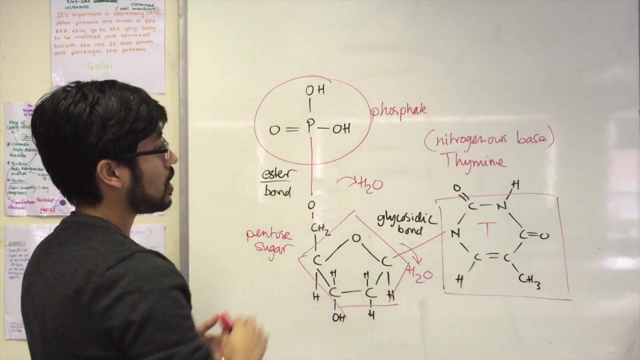 and I'll just draw the base With a kind of square shape. Okay, So there we have it. I'll rejoin you now when we discuss how these nucleotides can be joined together to form the polymer. Okay, remember, this is our repeating unit, the nucleotide. 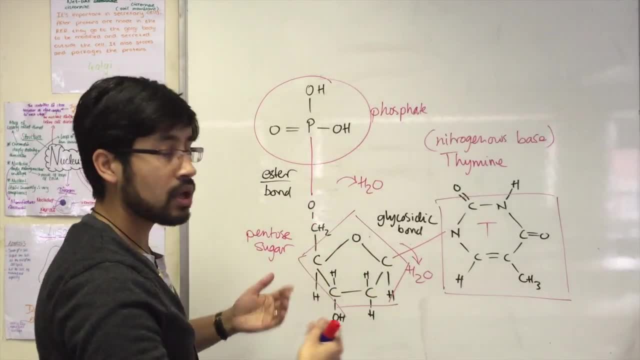 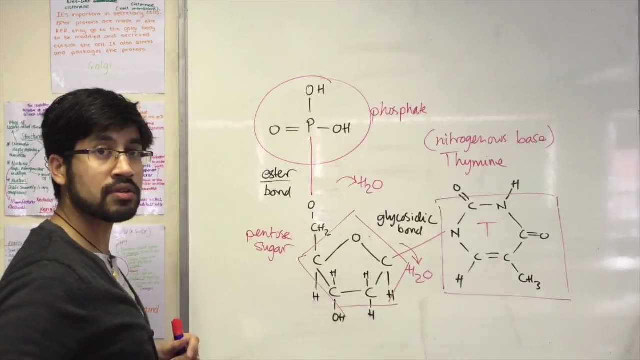 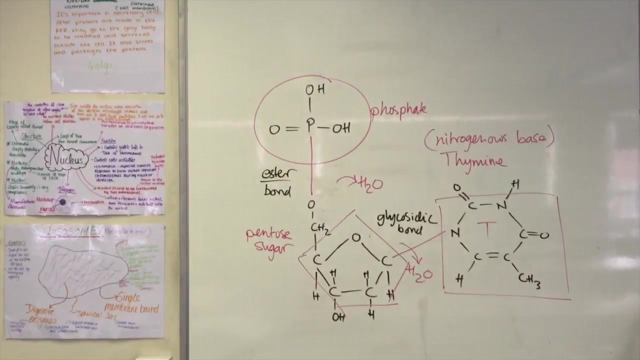 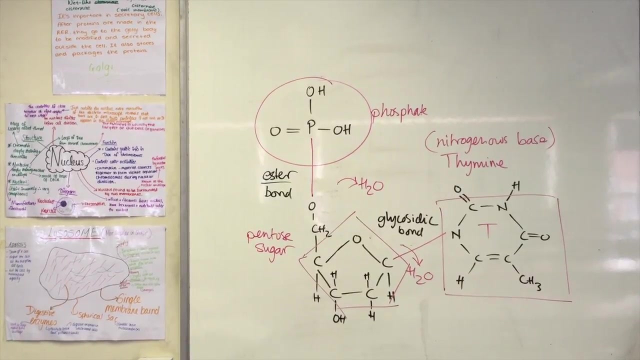 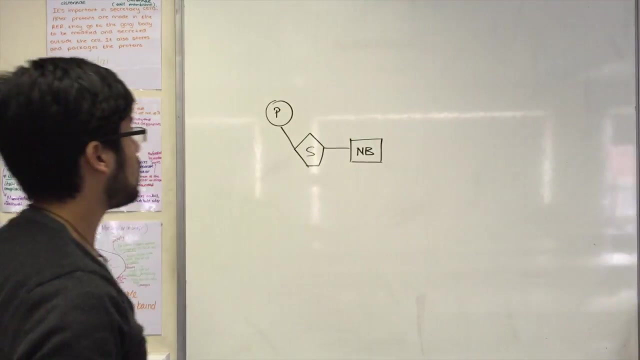 And this is going to be then joined again and again to form the polymer. Alright, And the polymer can be either DNA or RNA, but they're both made of nucleotides. Okay, See you in a bit. Alright, welcome back. 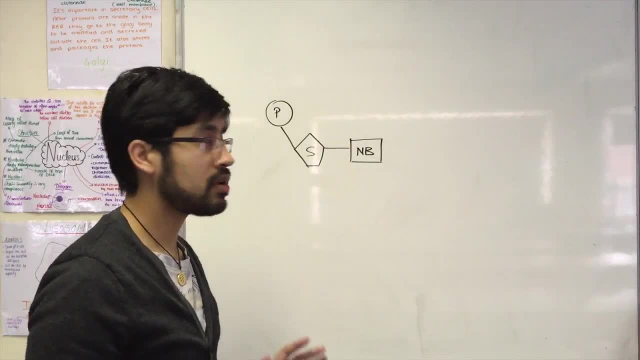 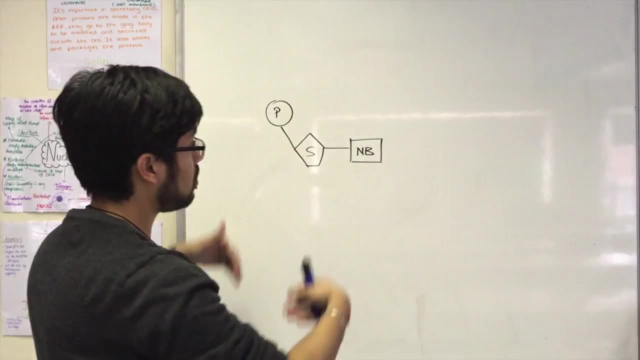 Right, so we discussed the detailed structure of the nucleotide just now. I'm going to simplify that now. I'm going to simplify that now to something like this, because as our polymer grows, it's going to become a bit more complex. 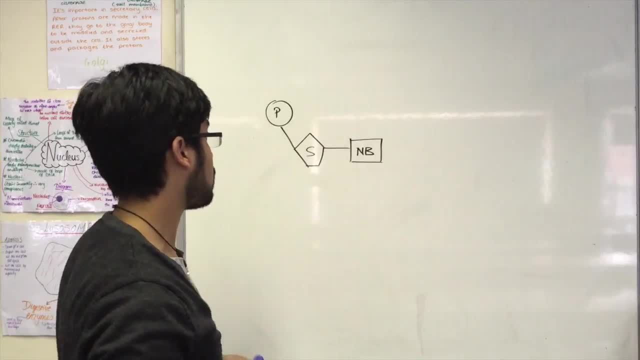 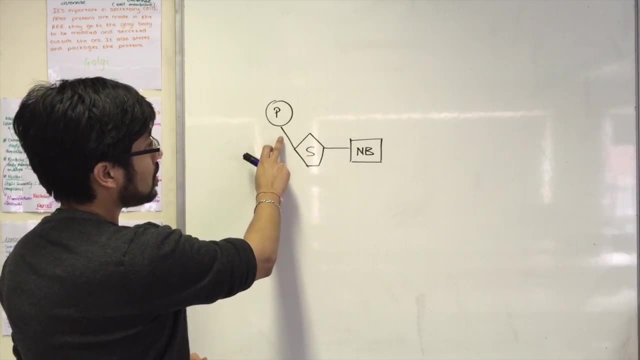 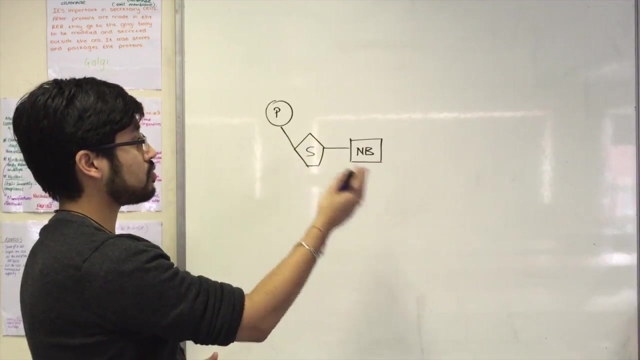 and it's not going to be convenient to draw all the atoms out. Okay, so here we have the same thing that you've just seen, just simplified: Phosphate group attached by the ester bond to the pentose sugar. It could be a ribose or deoxyribose. 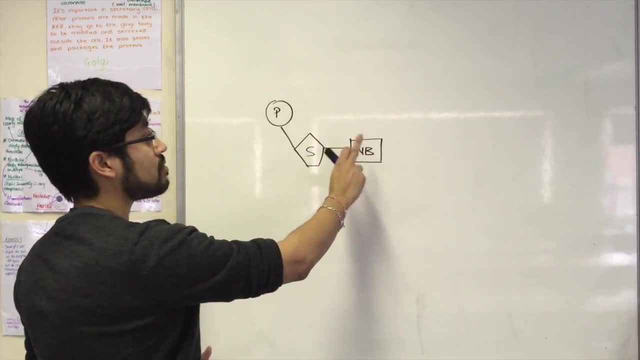 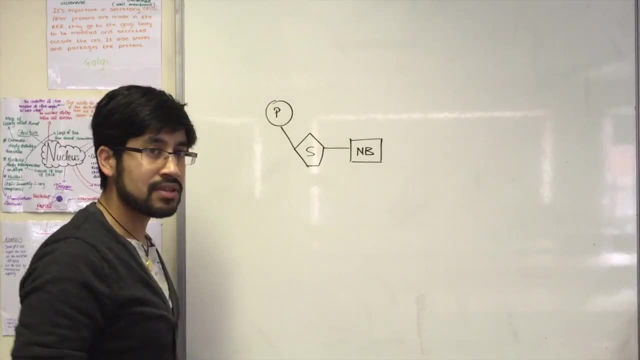 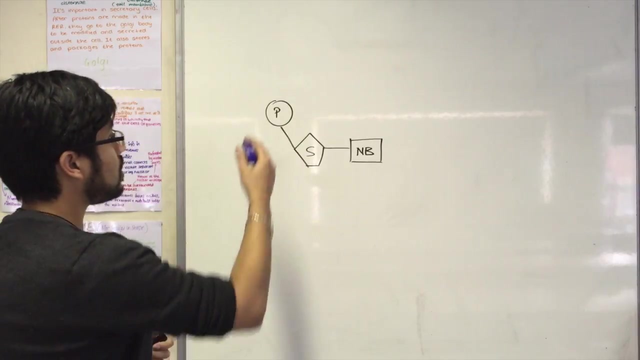 Pentose sugar. Pentose sugar, attached to the nitrogenous base by a glycosidic bond. Okay, Now what happens next is in the next level of structure. so, moving on from the monomer, what can happen is different nucleotides can line up and be joined together. 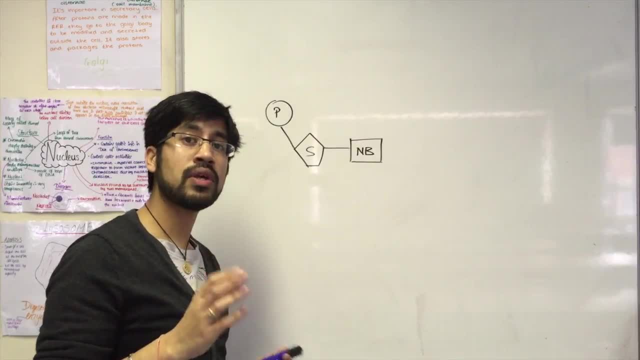 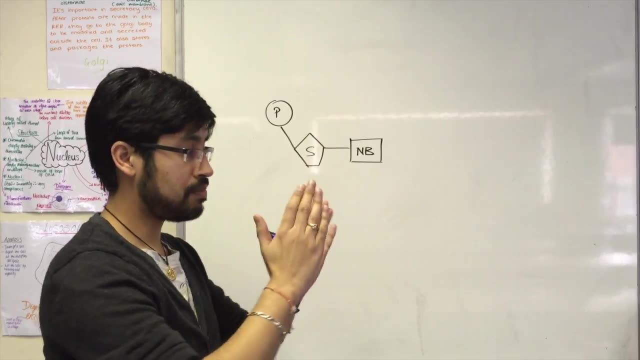 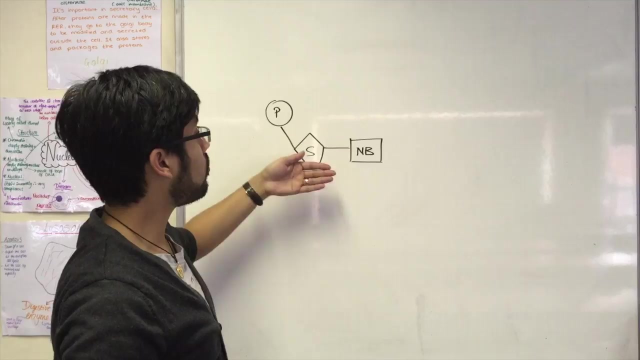 But this is not the same case as a carbohydrate. In a carbohydrate, you remember that it's always the same repeating unit joined end to end. But in the case of nucleic acids, you don't have the same nucleotide over and over again. 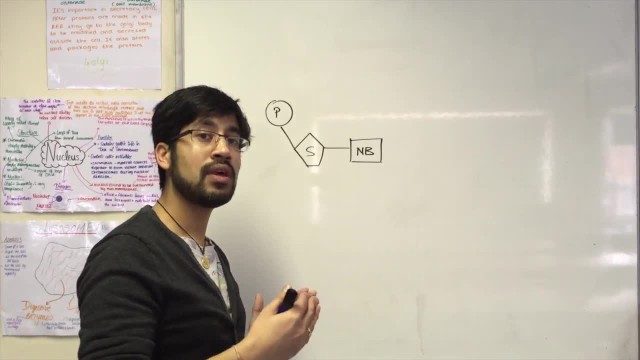 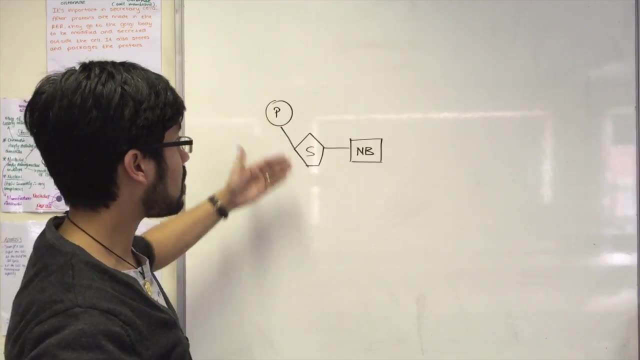 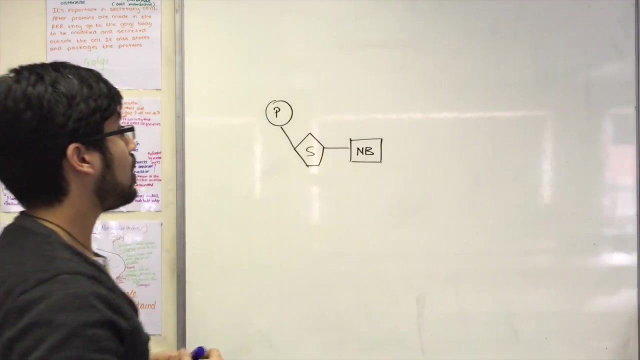 You have different versions of that nucleotide, And what makes the different versions of the nucleotide is not the phosphate or the sugar. They're always the same, But what you can have is different bases. Okay, Nitrogenous bases. Now, there are four nitrogenous bases. 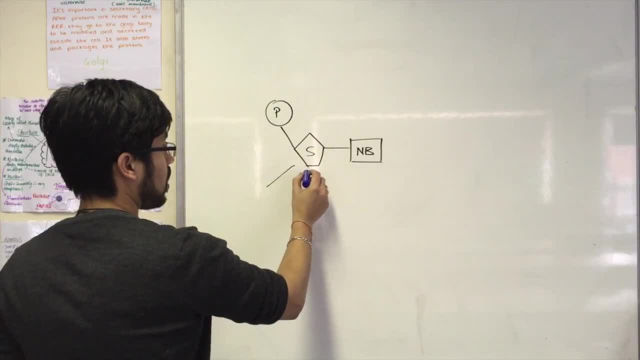 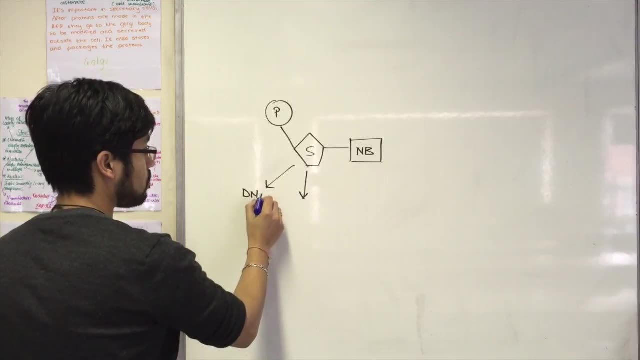 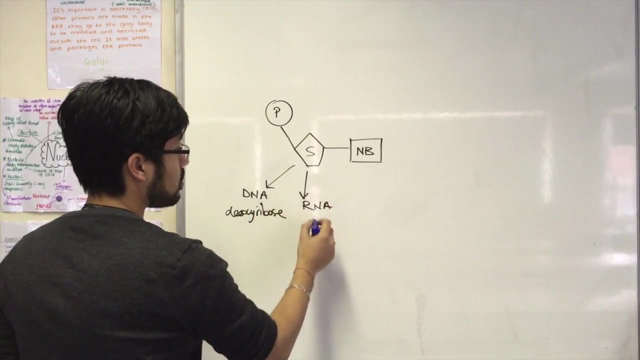 So let's just not get ourselves confused. The sugar can be of two types. If it's DNA, that sugar is going to be deoxyribose Always. If it's an RNA nucleotide, that sugar is always going to be ribose. 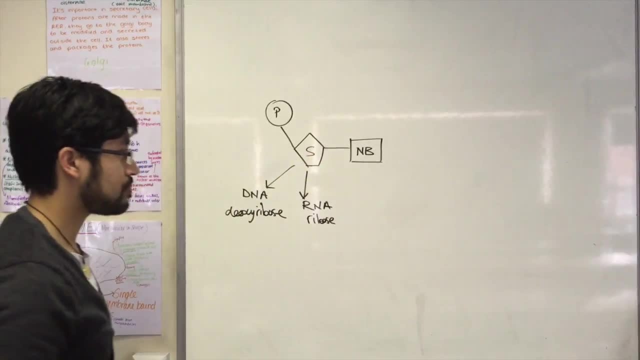 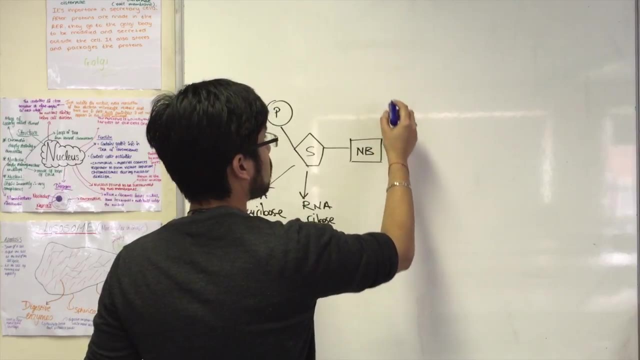 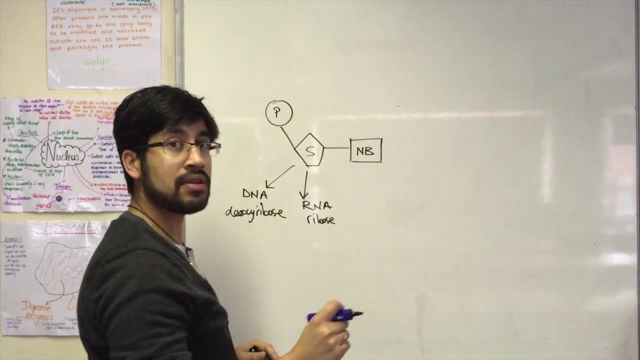 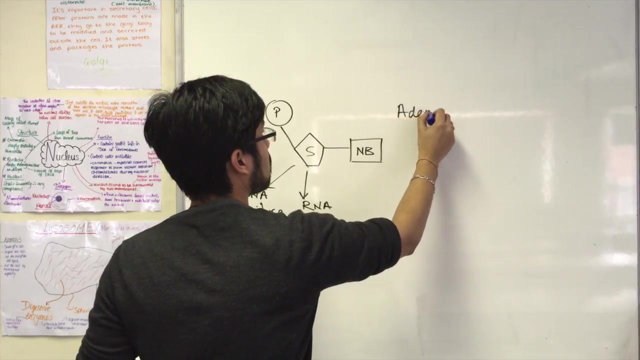 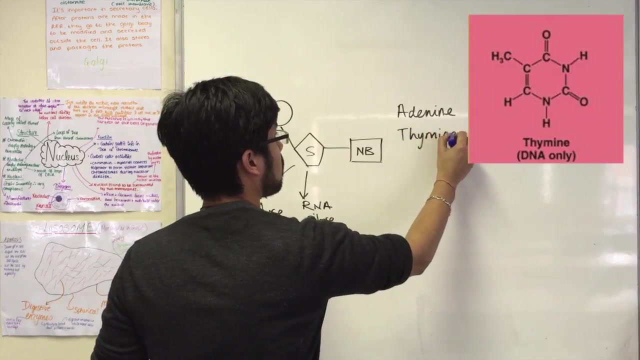 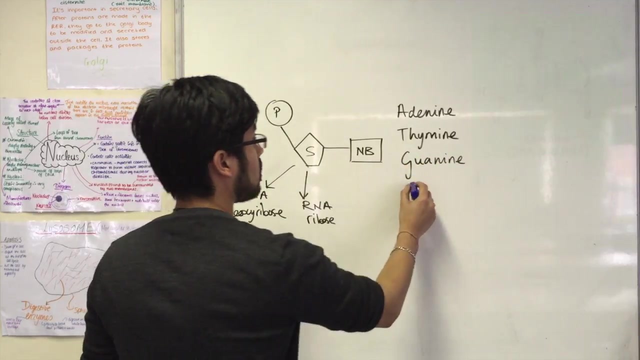 Okay, Now let's look at the bases. The bases are like this: There are four bases in each of these. Now in total, there's five bases In DNA. there is adenine, thymine, guanine and cytosine. 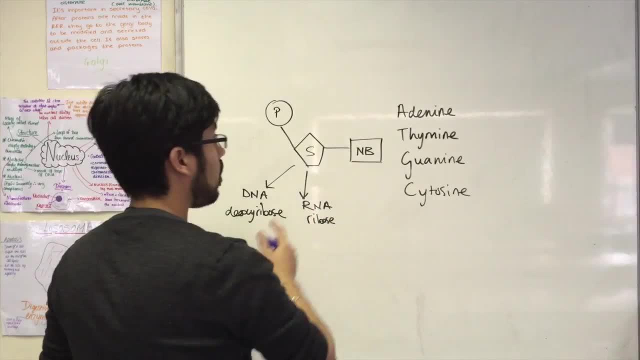 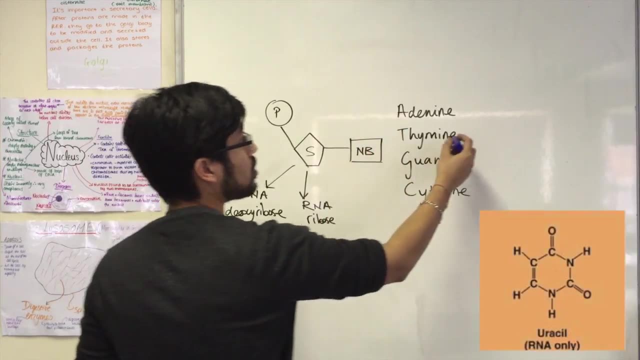 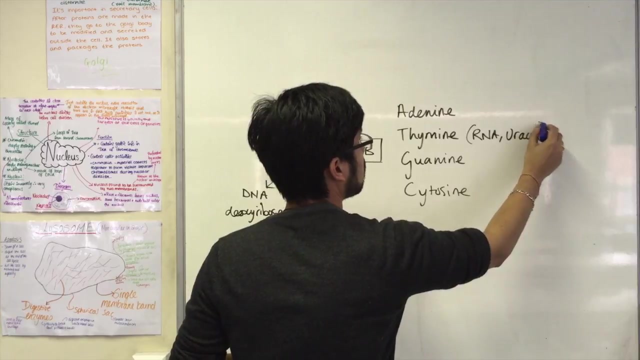 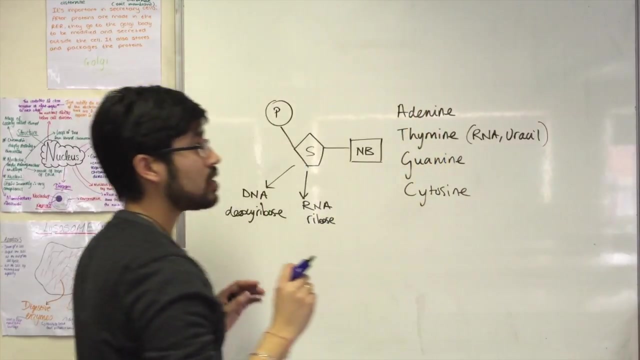 Okay. However, in RNA you don't have thymine, You have uracil. So what I'll do is I'll just put a bracket in RNA- uracil, not thymine. Okay, So in total there are one, two, three, four, five bases. 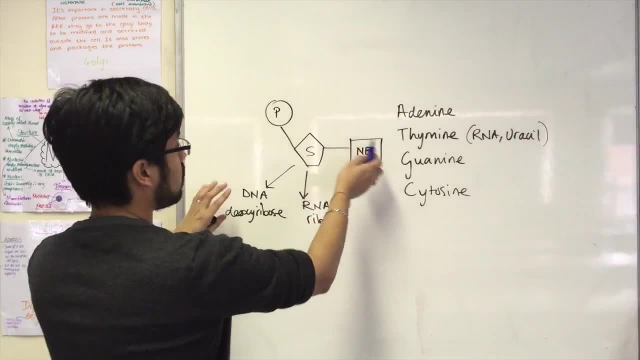 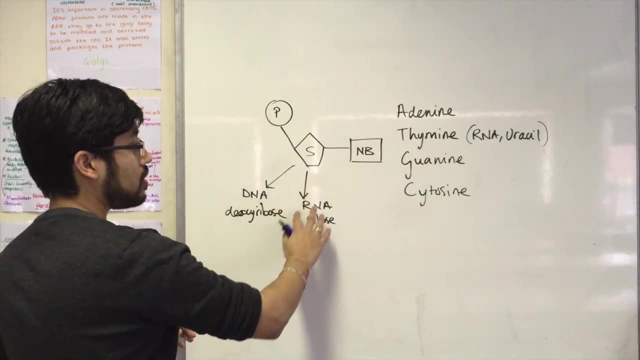 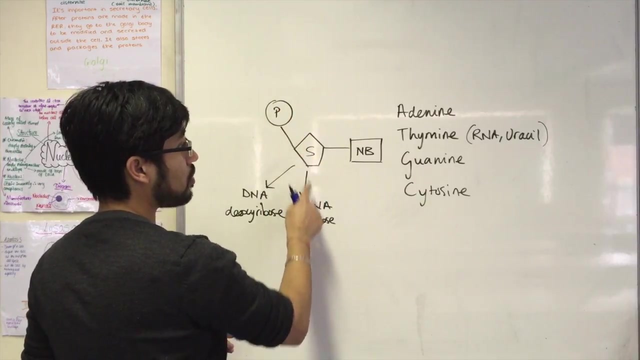 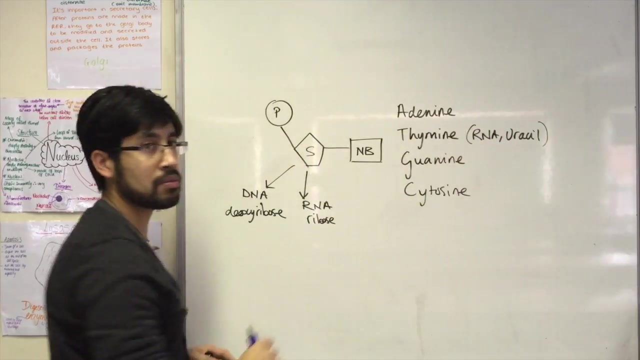 But all DNA nucleotides will have the deoxyribose sugar And these four bases, And in RNA the nucleotides will be phosphate and ribose sugar plus adenine or guanine or cytosine or uracil, not thymine. 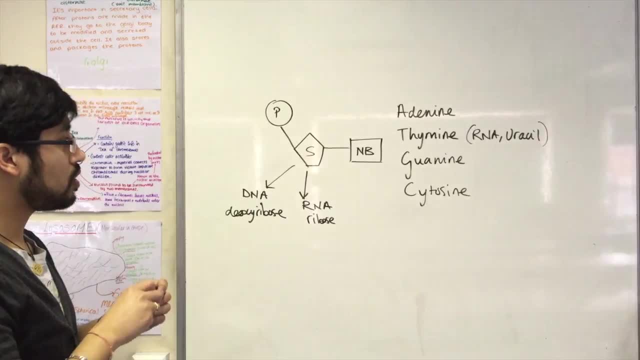 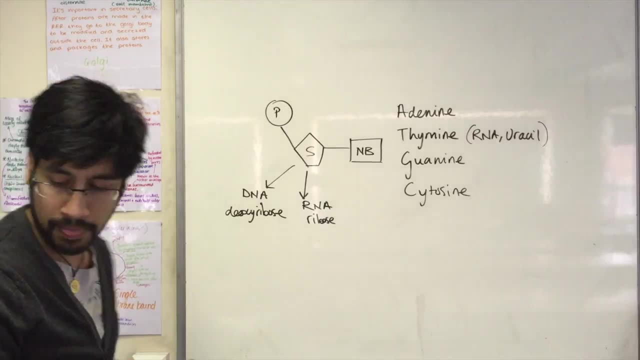 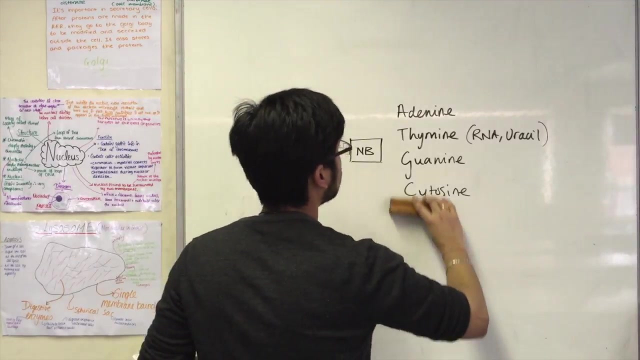 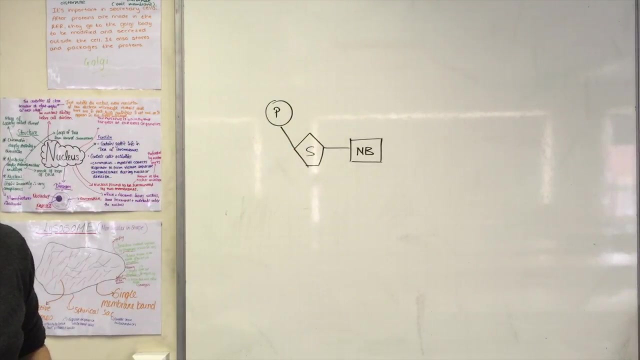 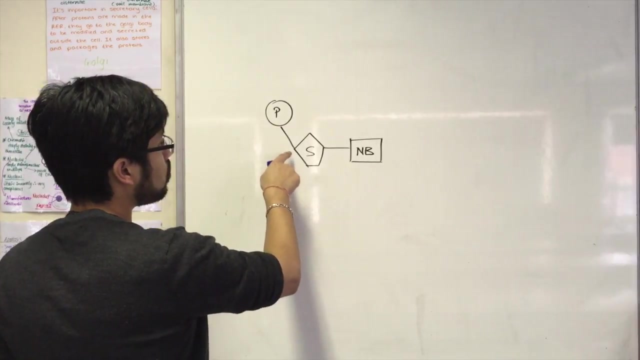 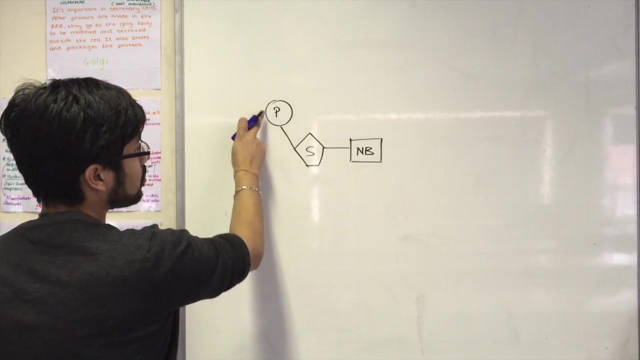 Okay, So this is the situation And we'll move on. We'll move on now. Okay, Right, So how does the polymer form? Well, you recall that these carbons had OH groups on them. One OH group was used to form the ester bond to this phosphate. 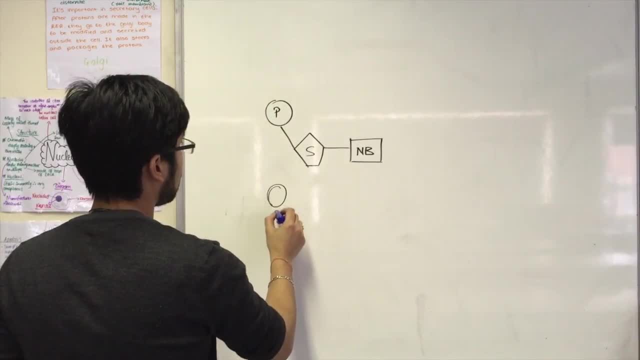 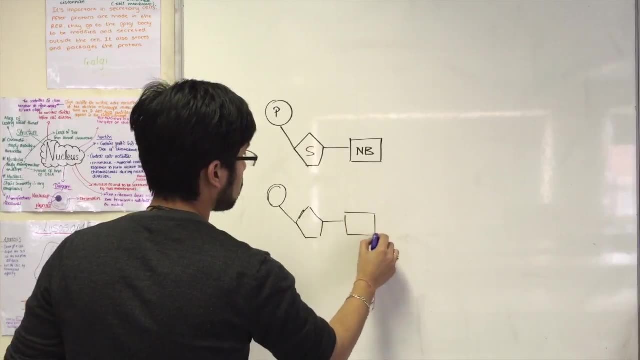 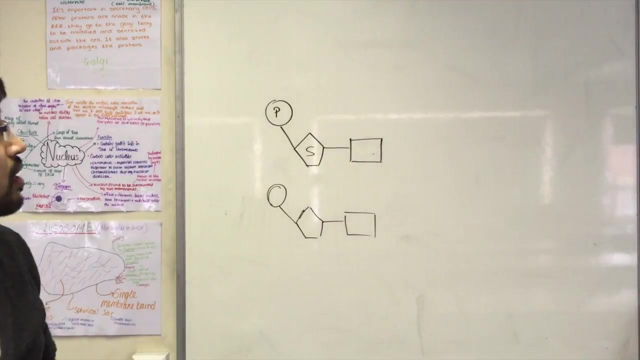 Now if we have another nucleotide lining up down here with its own nitrogenous base? Now let's get a bit more specific here. Let's say for the: in this example we're looking at a chain of DNA nucleotides. 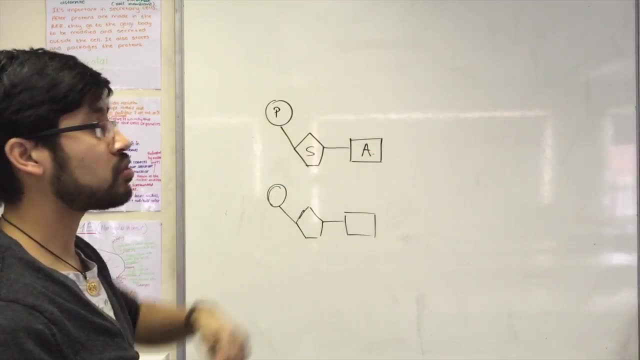 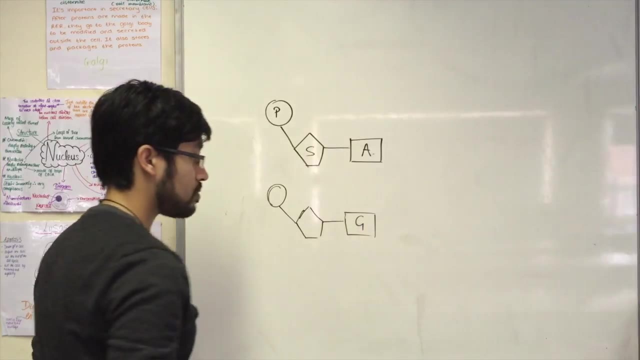 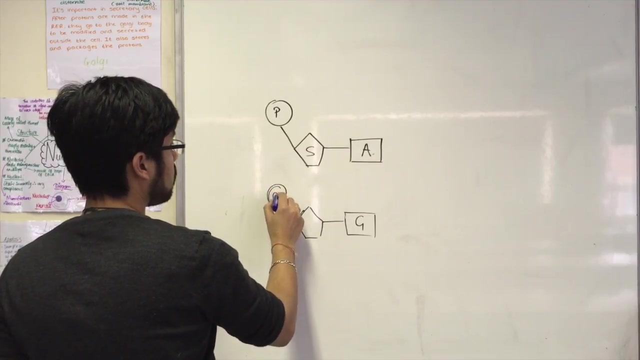 The first one might have contained the nitrogenous base. This one might have contained the nitrogenous base adenine. The next one might contain the nitrogenous base guanine. Okay, For example. Now what happens is that this phosphate group can form an ester bond. 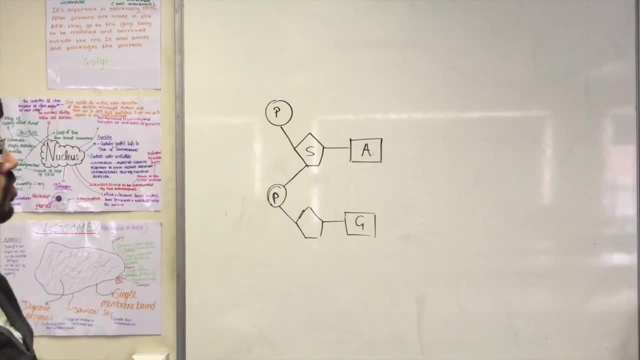 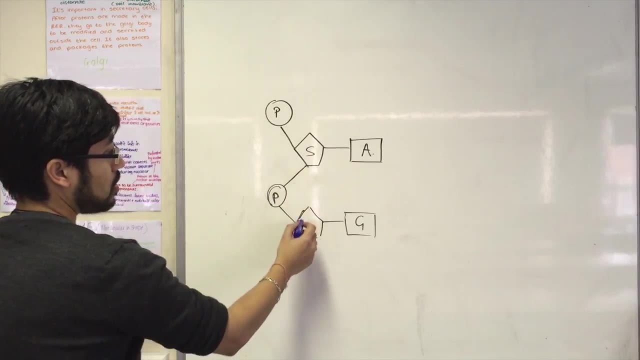 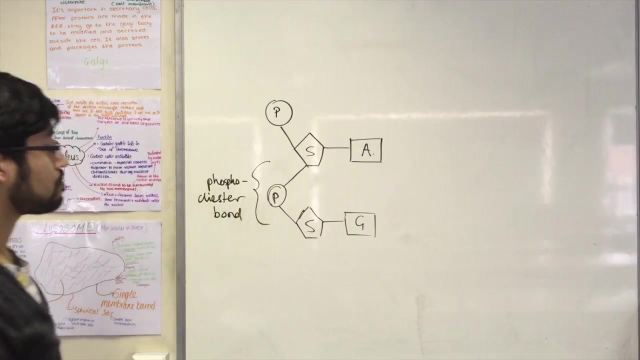 with one of the OH groups on the other carbons of the sugar. Okay, So now we have a phosphate group which has formed two ester bonds to two sugars. Okay, So this is now called the phosphodiester bond. Okay, 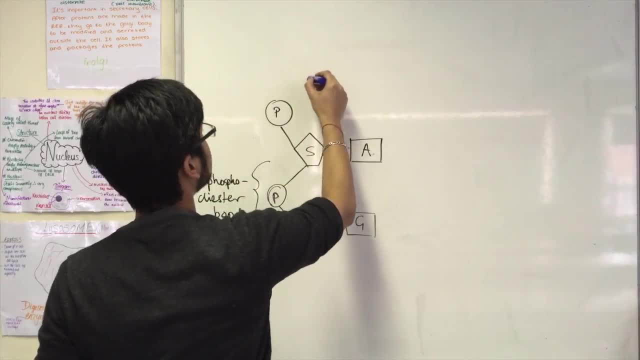 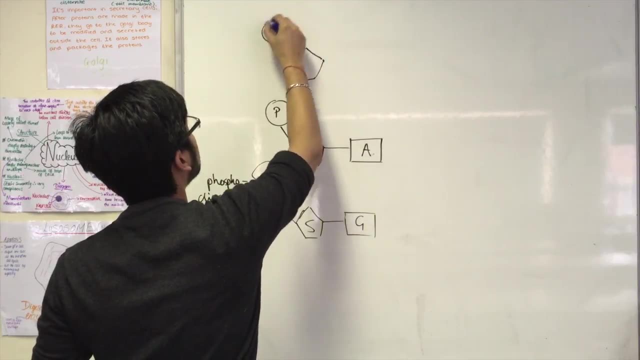 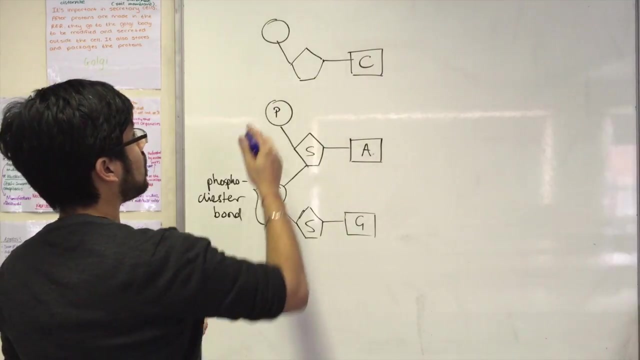 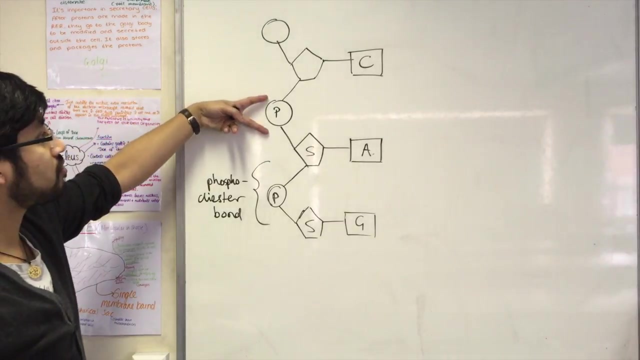 And this can happen many times. So we could have another one up here, And in this case it might be cytosine, And again the phosphate group can make a bond to the sugar over there- Another phosphodiester bond. 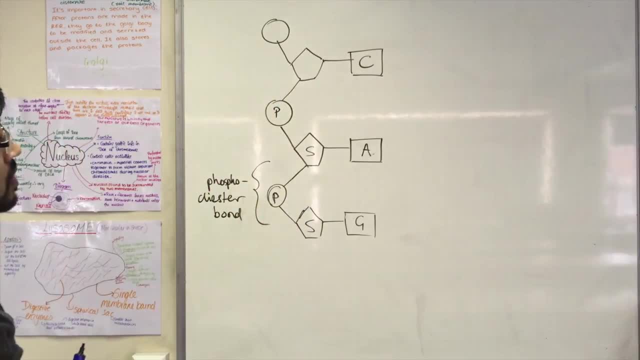 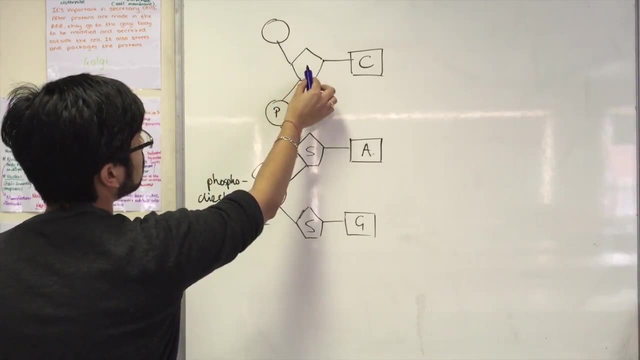 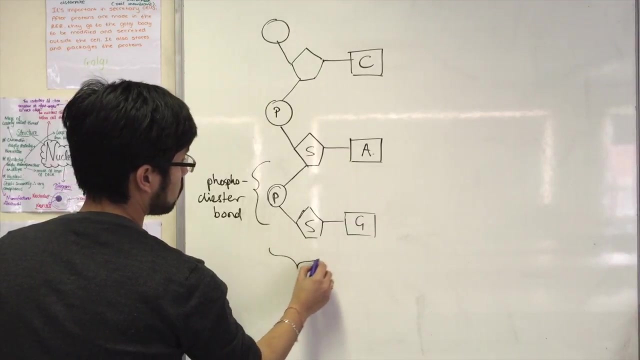 And thus what we will be constructing, if we carry on in this process, is what we call the phosphate-sugar bond, The phosphate-sugar backbone or the sugar-phosphate backbone. Okay, So if I just draw this there, 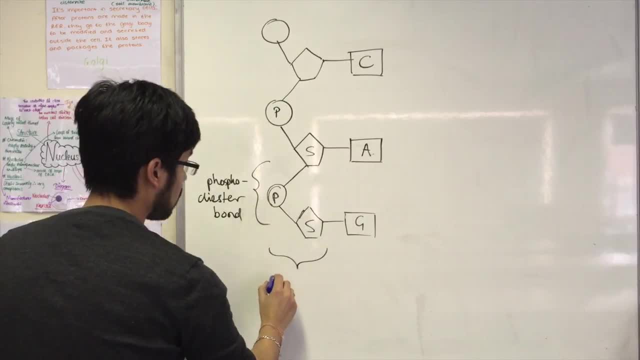 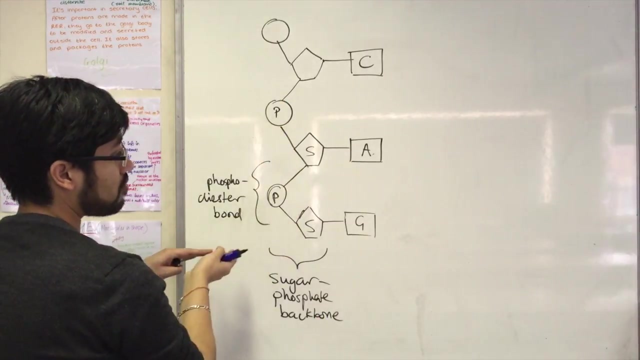 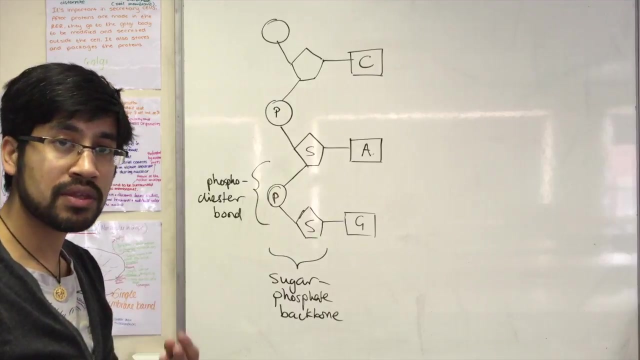 This. what we have here is the backbone, The sugar-phosphate backbone, Right? So this is the backbone, And what you have sticking out from that backbone is, or are, the nitrogenous bases. Okay, And it's, you know, the sugar-phosphate-sugar-phosphate-sugar-phosphate. 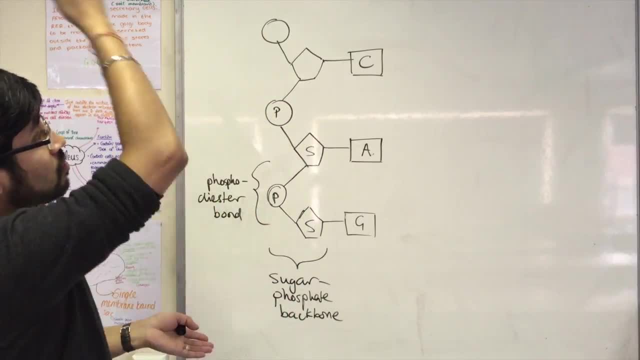 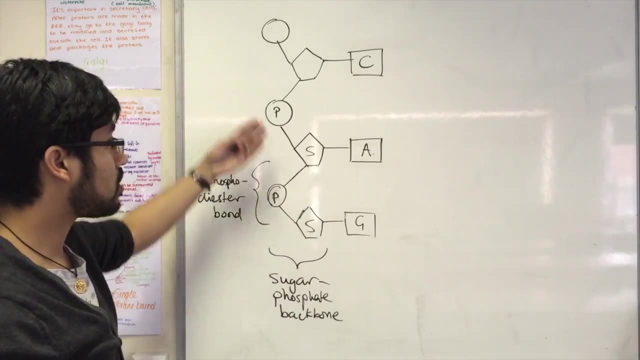 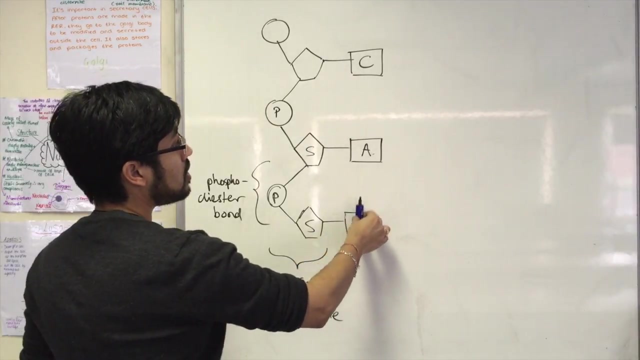 There's nothing unique about that. That's just a repeating unit all the way along. But what does give each polynucleotide its kind of unique identity, and the reason why it can act as information storage, is that you then develop a very unique sequence of these nitrogenous bases. 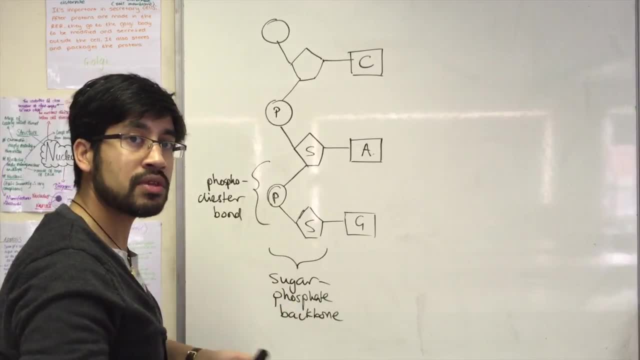 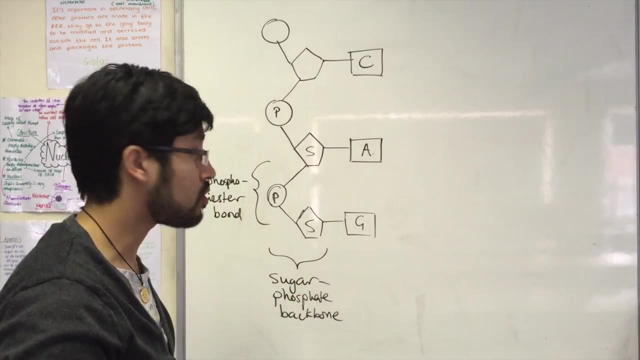 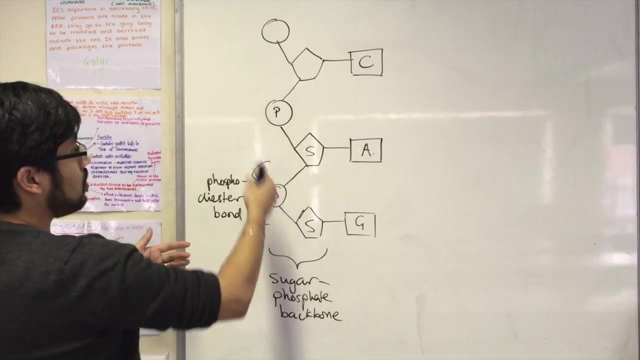 Okay, And depending on that sequence it can give you know it can be a way to store information And how that information is used. we'll look at that later on. Okay, So I hope you can appreciate now that suddenly we have the joining of separate nucleotides. 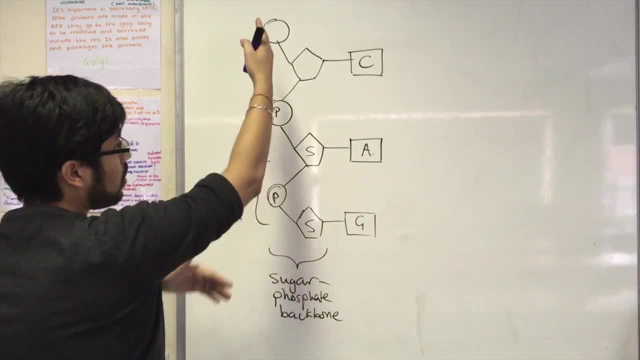 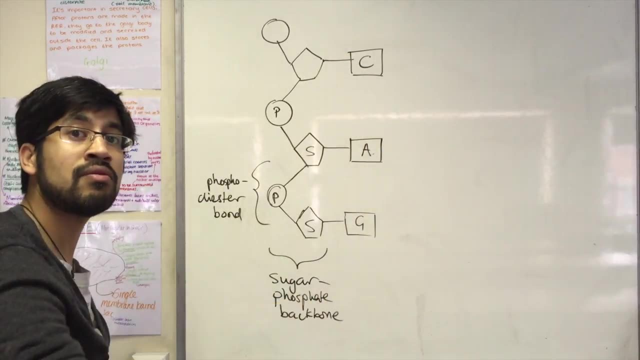 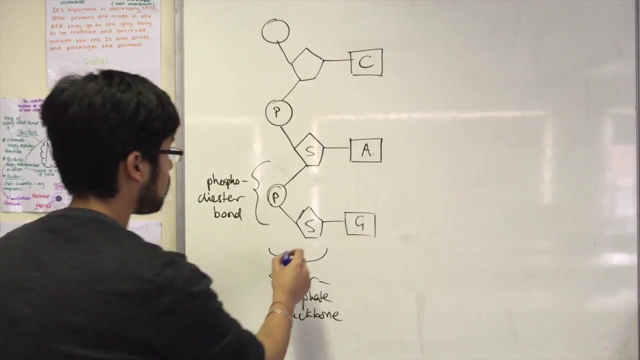 we have the formation of phosphatidase bonds, forming the sugar-phosphate backbone, and then we have a particular sequence of nitrogenous bases then developing along that chain of nucleotides. Okay, So let's just finish this off, So this could continue. 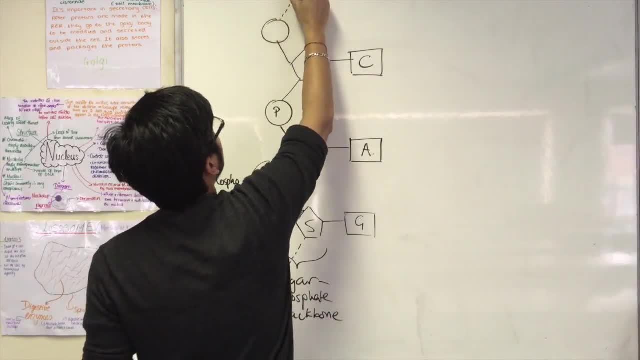 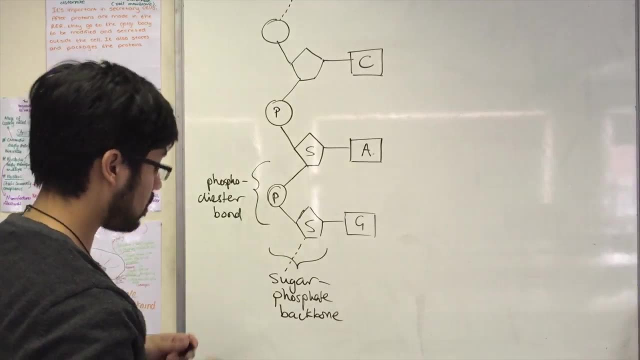 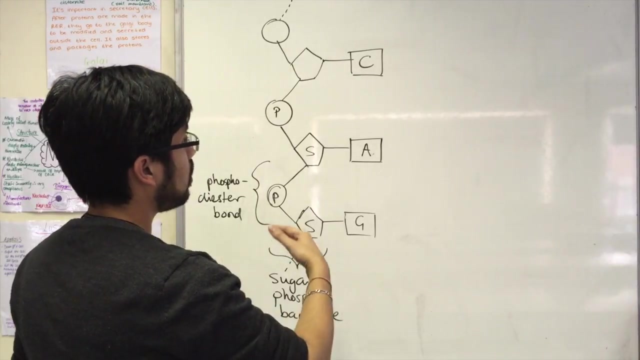 And you know, we could get a continuation up there as well. Right, So this could be just one segment of a DNA strand, But that's not the complete structure of DNA. Okay, Because what you have is the opposite strand. 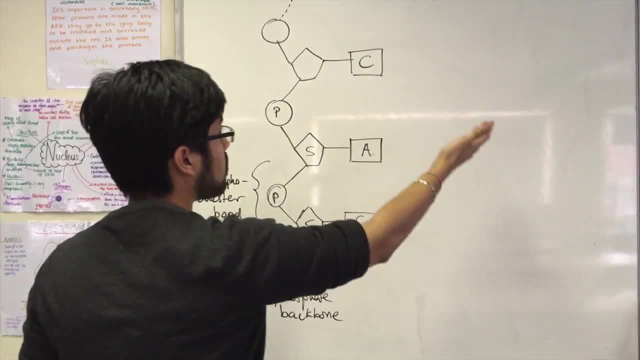 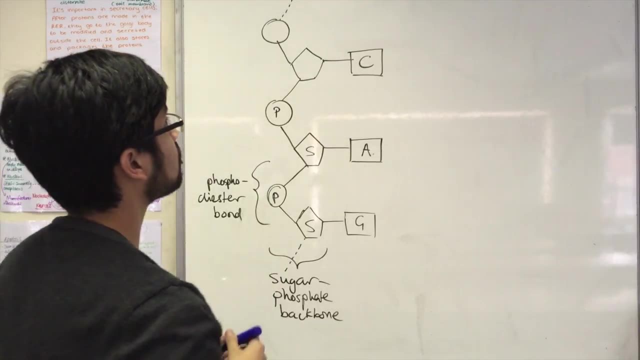 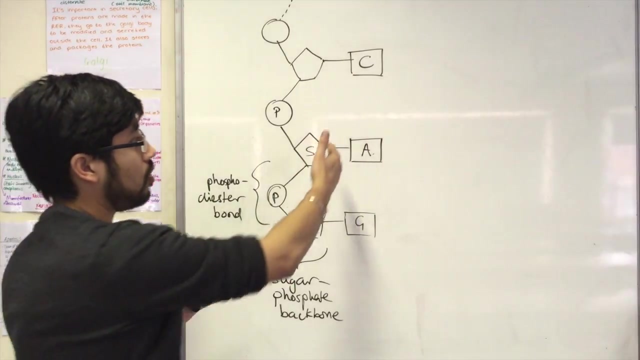 So, just like you've got a strand here, you'll have another strand which base pairs with this one. Okay, So what will happen is that these bases have groups on them that can form hydrogen bonds, So they bond with another base. 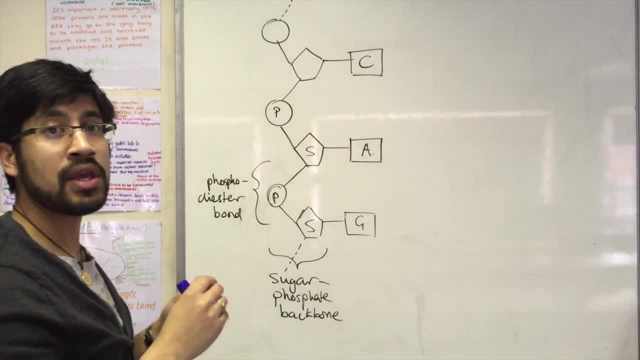 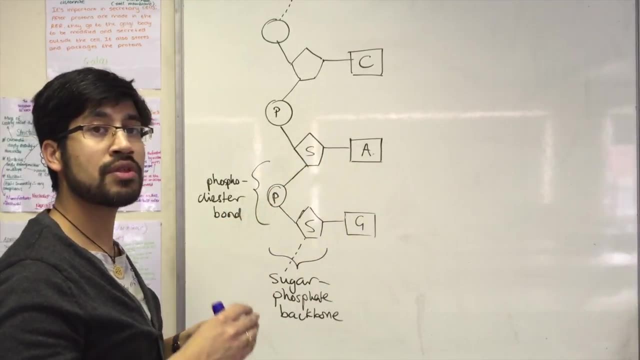 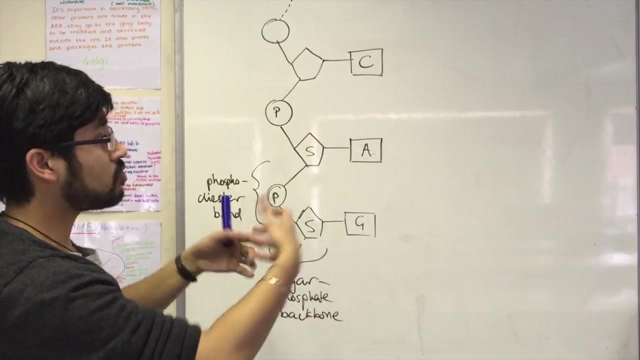 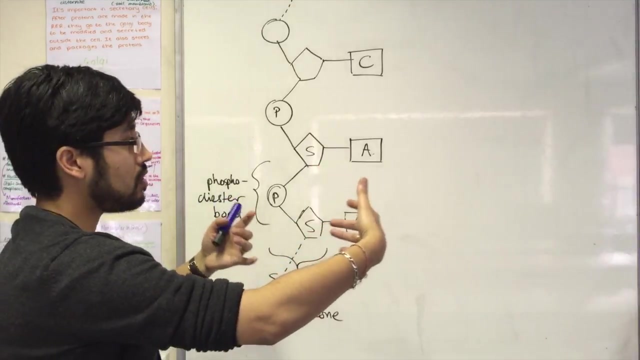 Now what happens is that cytosine always base pairs with guanine And adenine always base pairs with thymine, Simply because they have a shape that is complementary. Okay, They have OH groups in such a way that when they come close to each other, 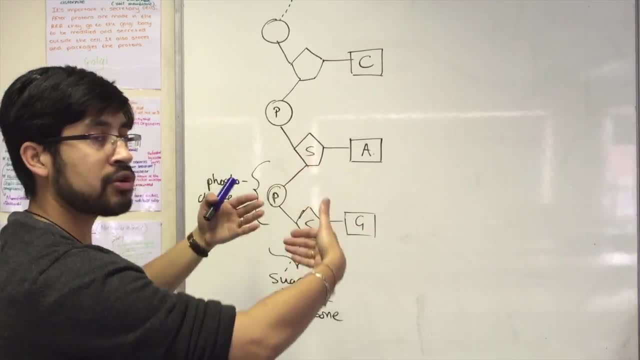 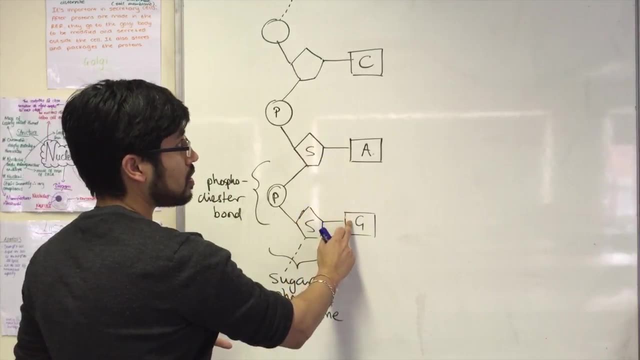 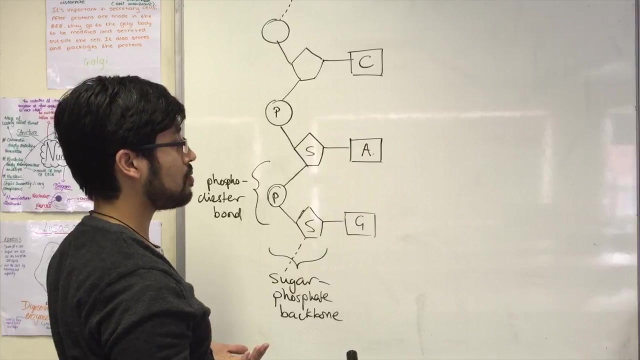 the partial positives and the partial negatives align with each other. Now, this isn't the case between adenine and guanine, And this isn't the case between cytosine and adenine, for example. Okay, But this is the case that whenever you get an adenine base, 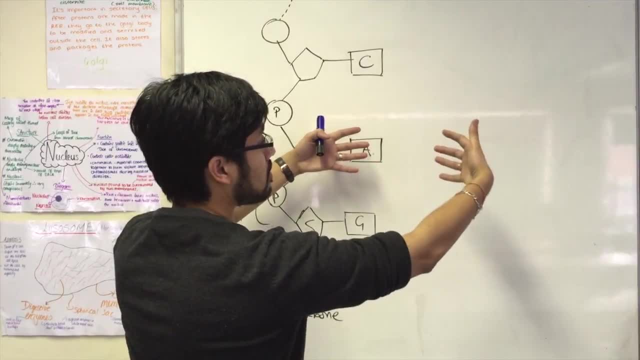 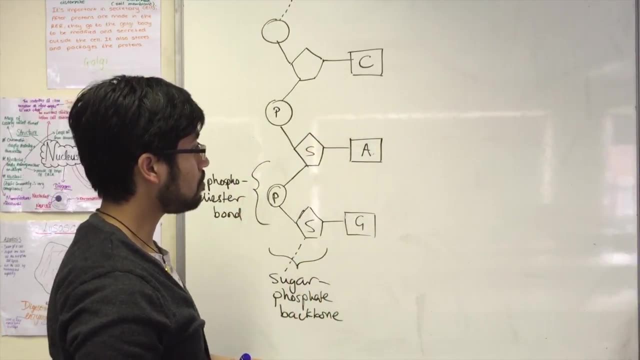 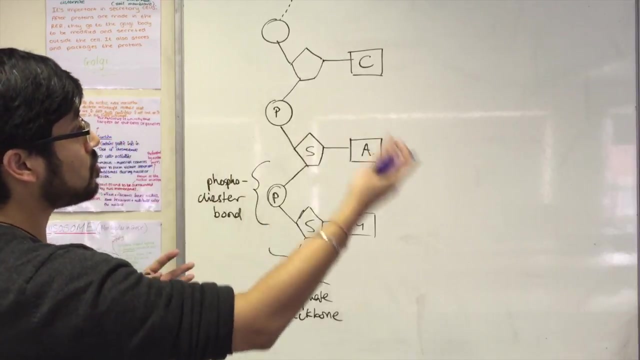 nitrogenous base and whenever you get a thymine base, they will align up so that they will form hydrogen bonds between each other. Okay, So if this happens, if this happens, what you get is you get other nucleotides floating around. 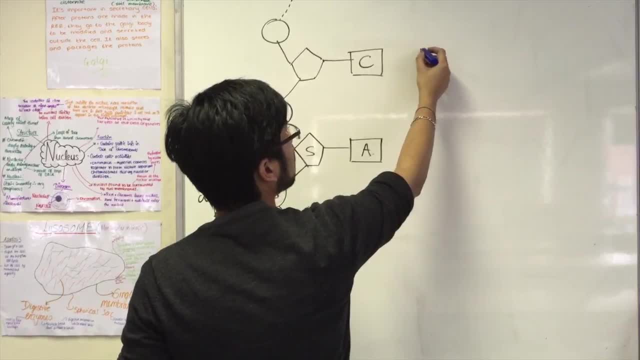 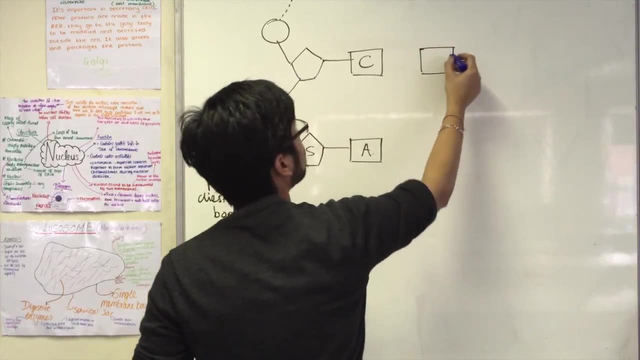 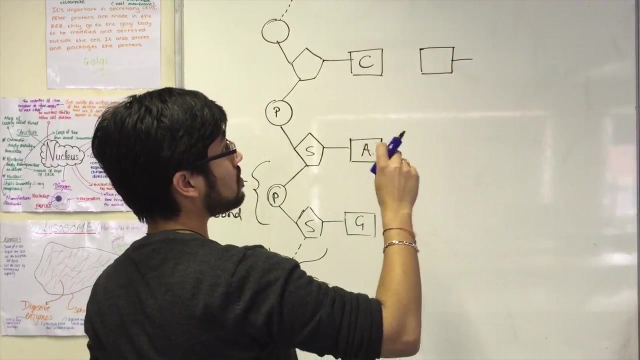 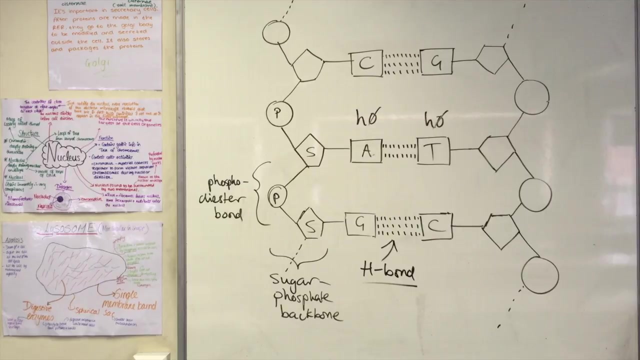 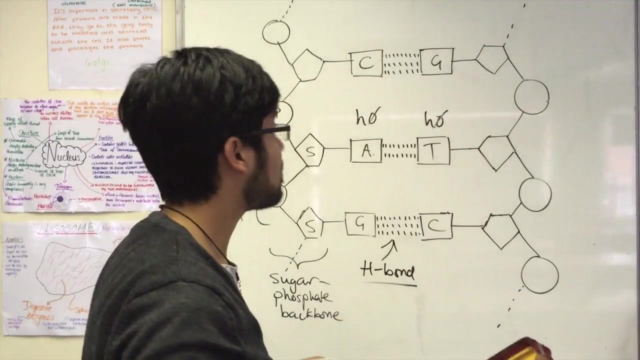 and they will base pair via hydrogen bonding. Okay, So if I had another nucleotide and that other nucleotide had guanine as its nitrogenous base, it will. Guys, I was talking for about 10 minutes and just realised that it wasn't recording. 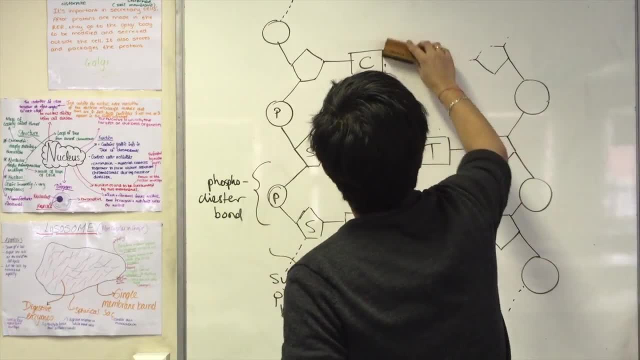 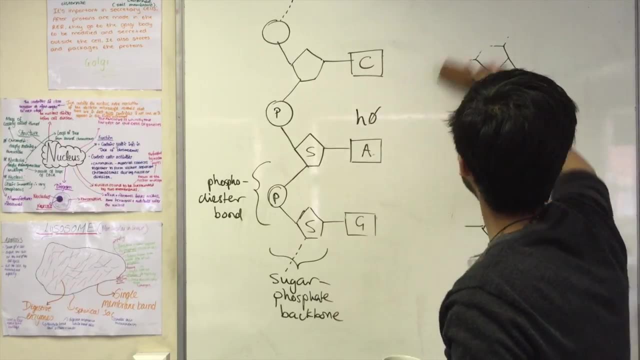 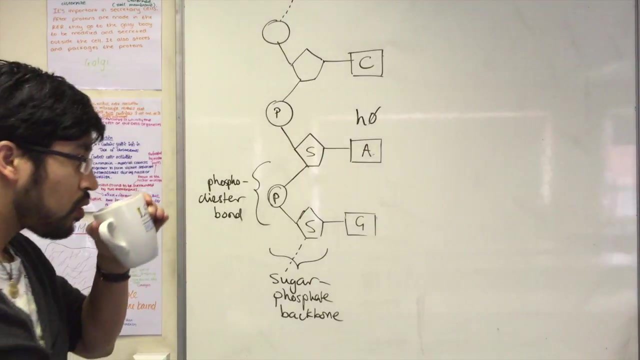 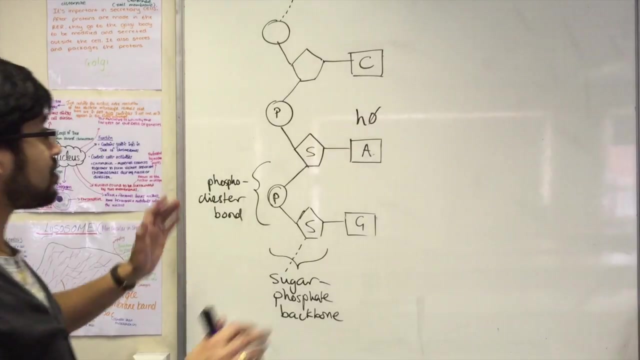 so I'm going to have to do it again, But that's life. Struggle is real, you guys? Right. here we go again, Right? So, as I was saying, this is just half of the structure of DNA. 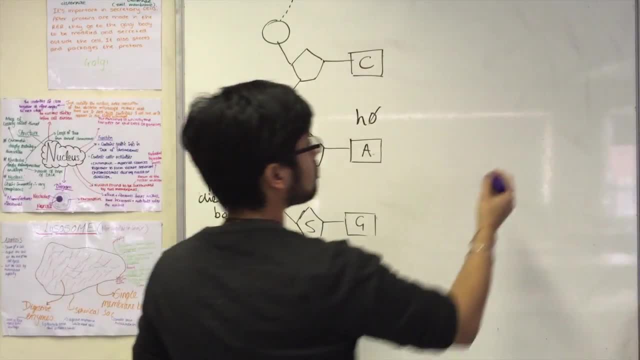 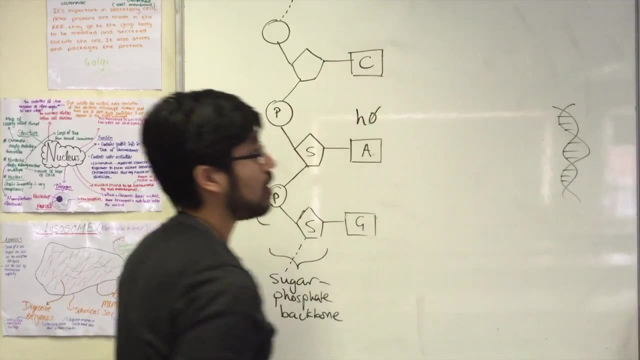 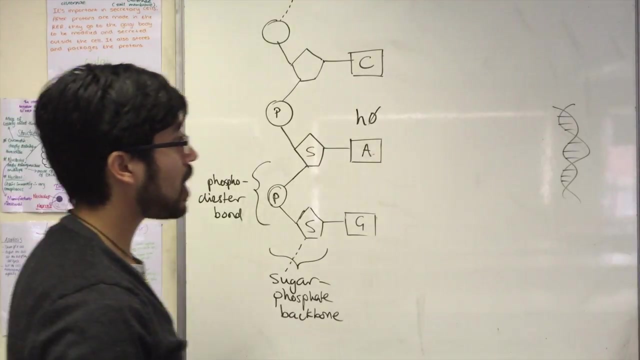 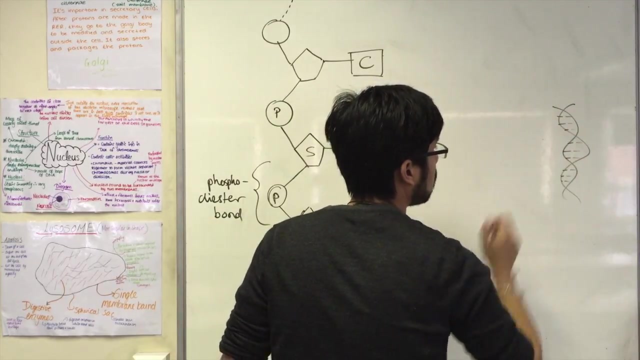 What it has also, as you know, the iconic diagram shows that there is actually two strands in DNA, and what we're going to look at now is why that is Okay. Why is it that there are two strands? What's holding them together? 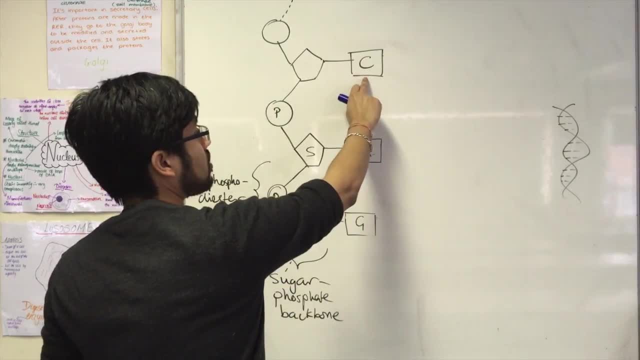 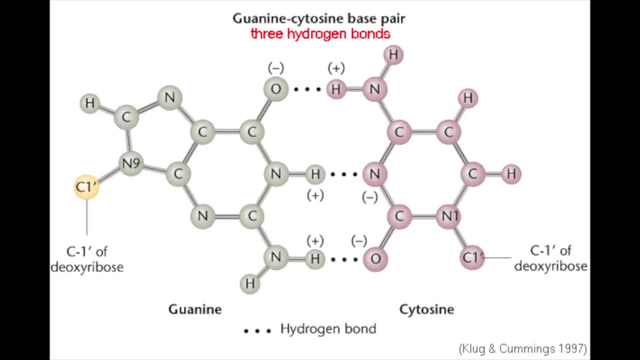 So what's holding them together is the interaction that one base can have with another one. So one base can have partial positive and partial negative regions, And what occurs is that if two bases are complementary to each other, ie if their positive and negative groups- 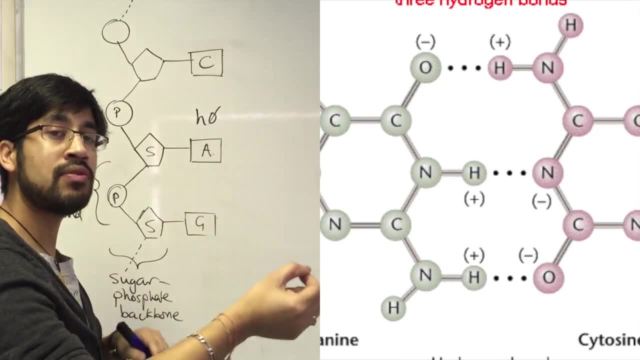 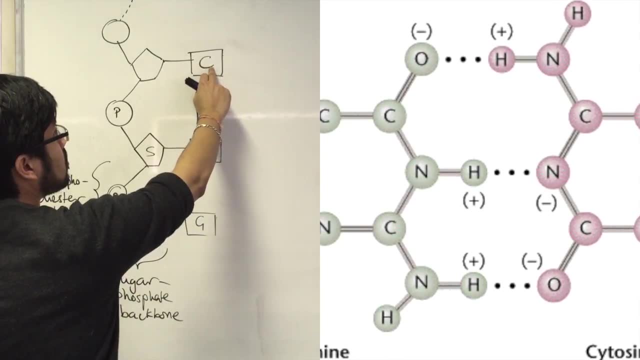 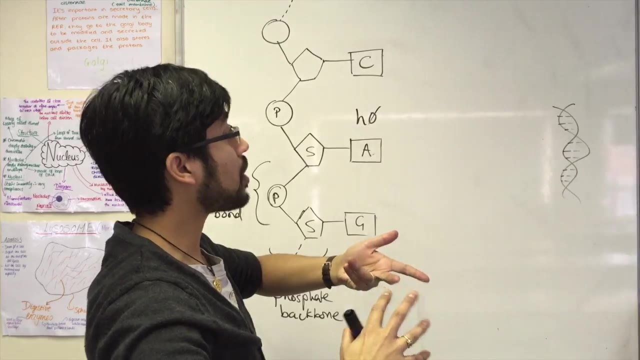 align with each other. they will form hydrogen bonds with each other. Okay, Now, this doesn't occur between cytosine and adenosine, Because the shapes of those molecules are not complementary to each other. Okay, Their negative and positive partial charges. 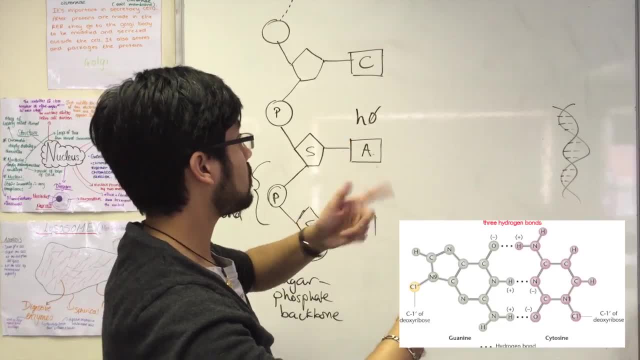 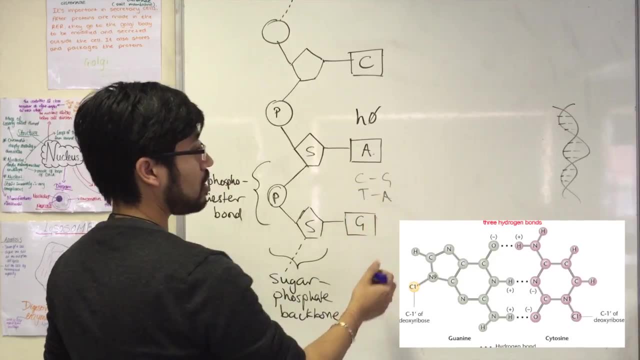 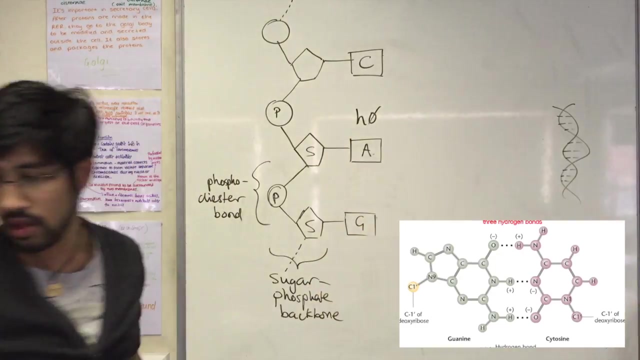 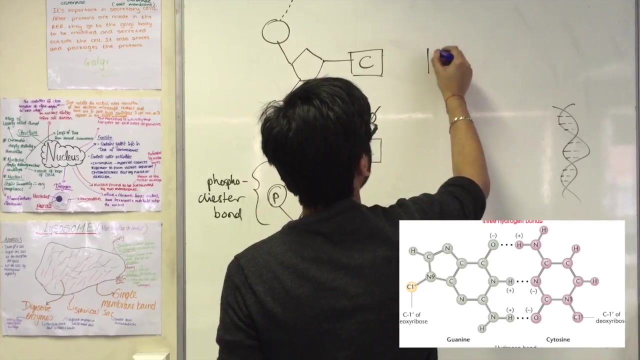 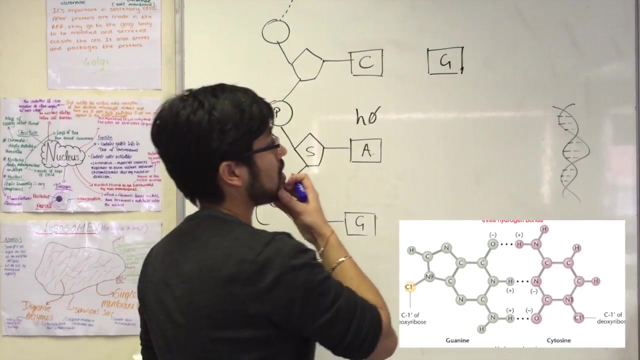 don't match up with each other. However, it does occur between C and G and T and A and vice versa. Okay, So if I had, If I had a G base, or if I had a nucleotide with a guanine base attached to it. 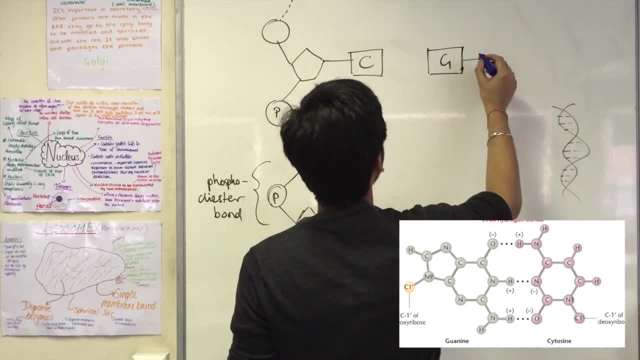 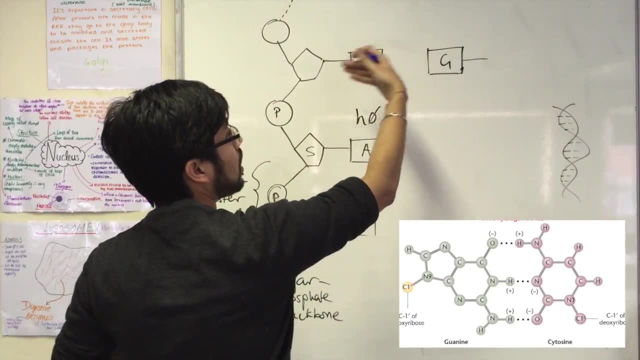 nitrogenous base, then it might float around for a little while but eventually it would, you know, come in the area of cytosine and align with it. It would pair up The hydrogen bonds between the two, would lock that guan. 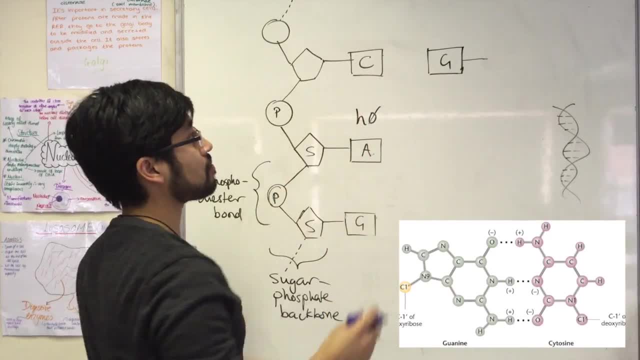 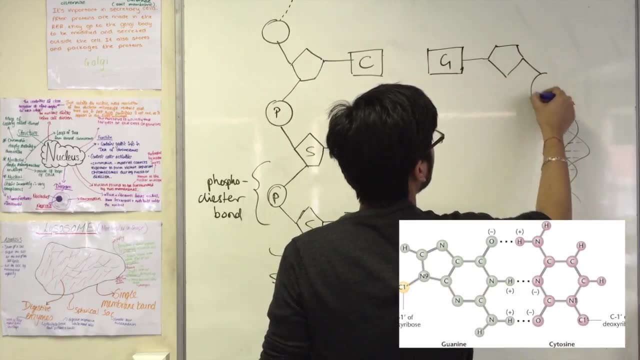 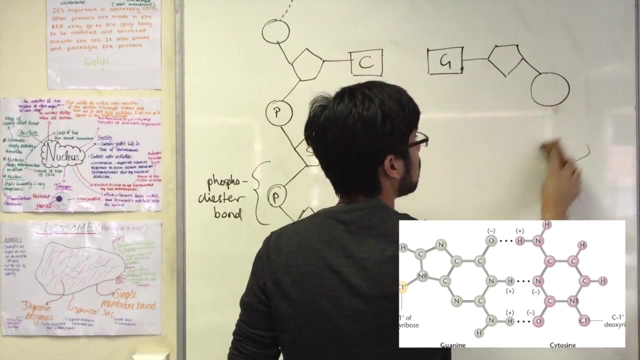 that guanine nucleotide in place, Okay. So the other thing you'll notice is that this only happens when the other nucleotide is in the opposite direction. Okay, It's in the opposite direction. That's when the C and the G 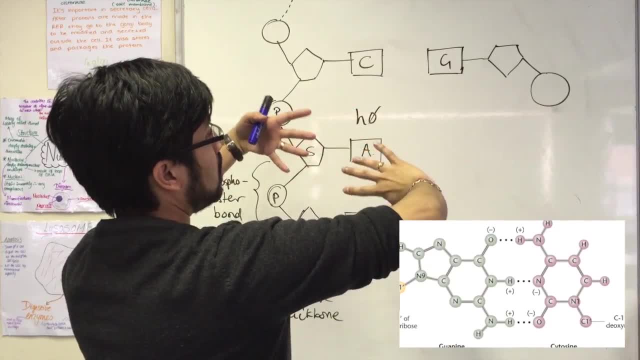 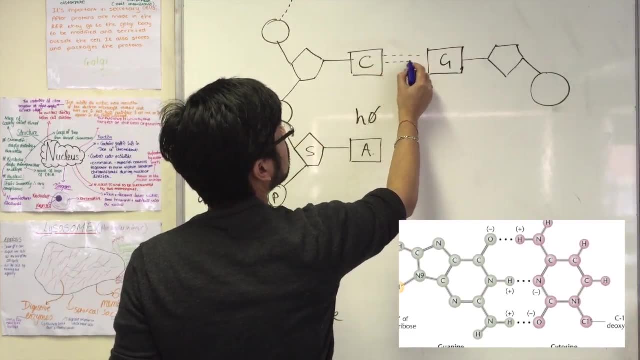 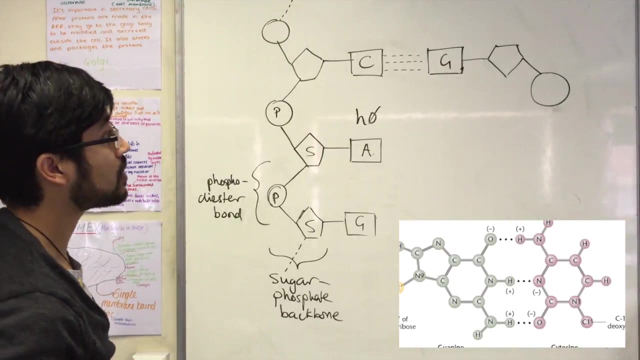 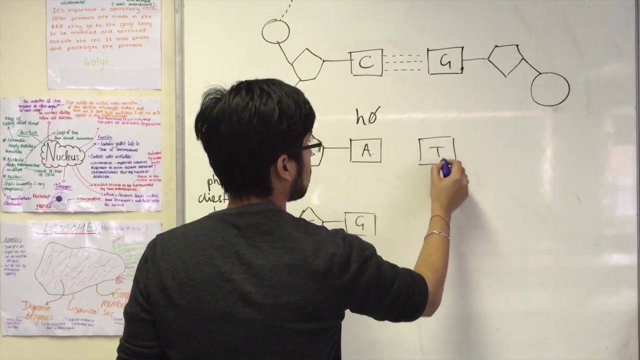 have a complementary interaction of hydrogen bonds. The other thing you need to know is that C and G form three hydrogen bonds between them. Okay, C and G form three hydrogen bonds between them. Now, if by chance, there happened to be a T nucleotide around? 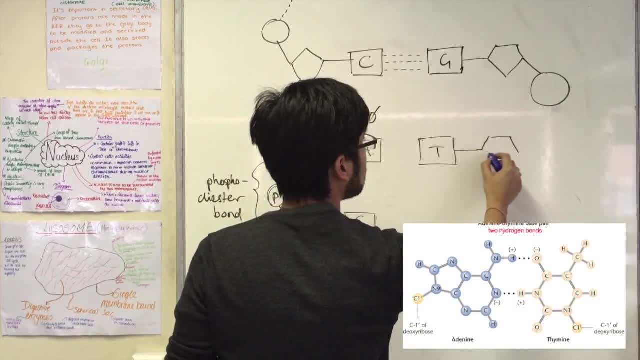 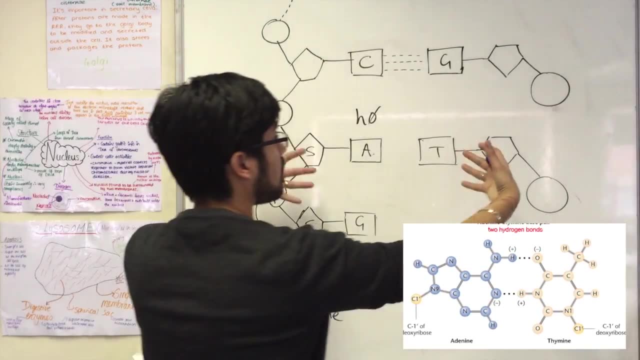 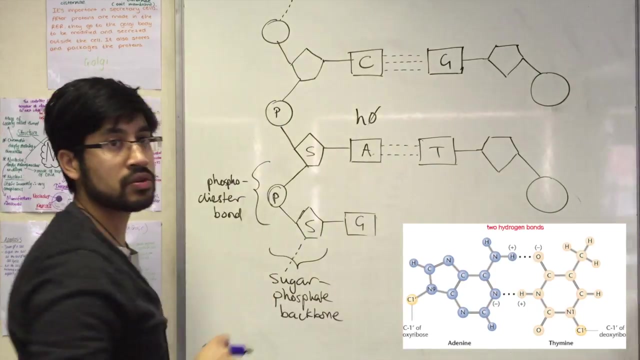 then a similar thing would happen when it lined up with an adenine nucleotide. Okay, In the same way it's flipped around, and when that happens, their partial positive and negative charges line up and they between them form two hydrogen bonds. 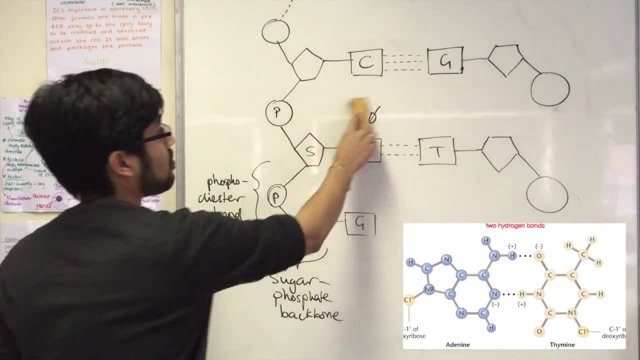 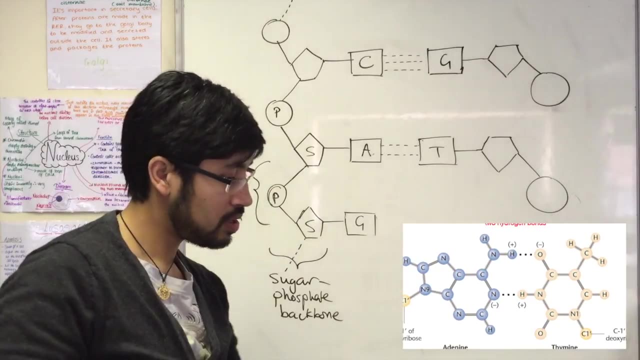 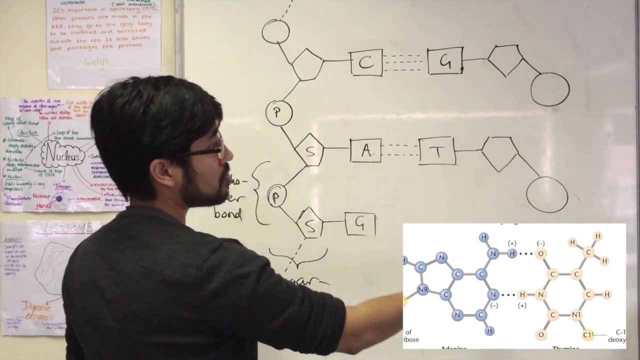 Okay, Let's just get rid of that for now. They between them form two hydrogen bonds And in this way, if you have a very long strand- and you do- you only need that one strand and the other strand will just start. 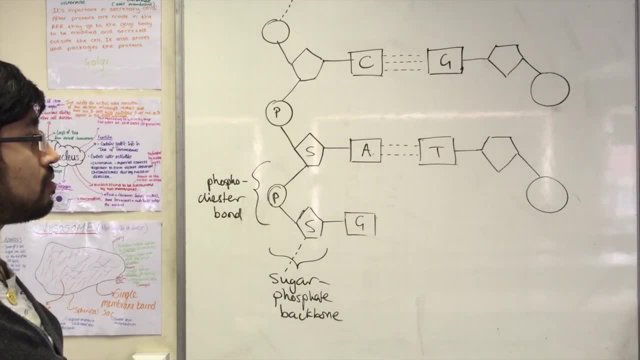 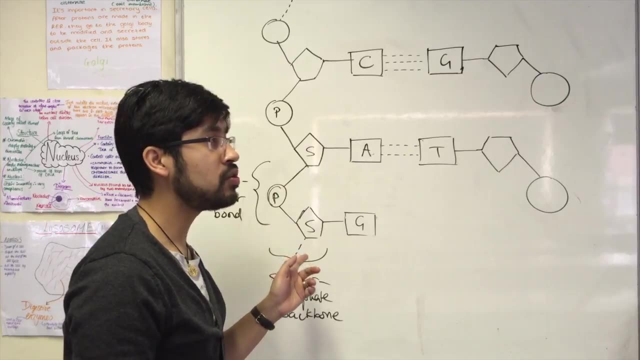 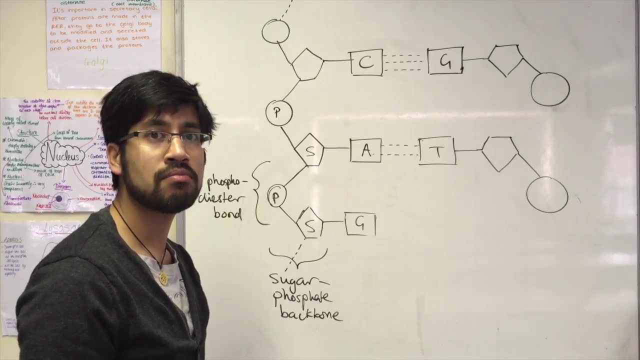 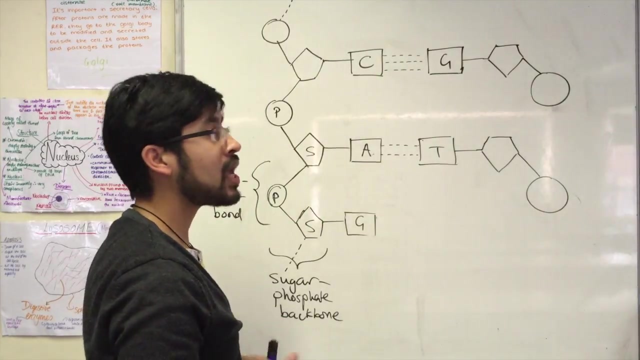 forming itself. Now, this is very lucky, because if you had one strand, you could make two. Maybe you could duplicate your DNA, Right, Pretty cool. Maybe that might allow organisms to replicate their genetic information, and I don't know. 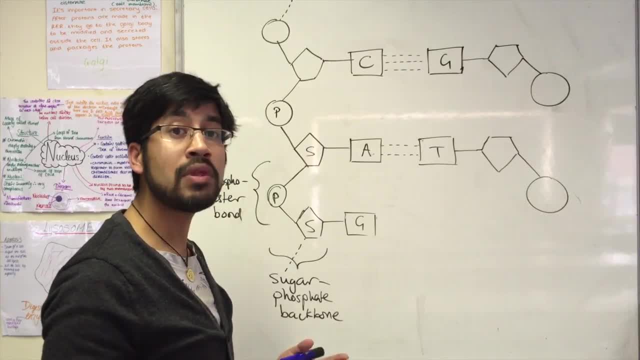 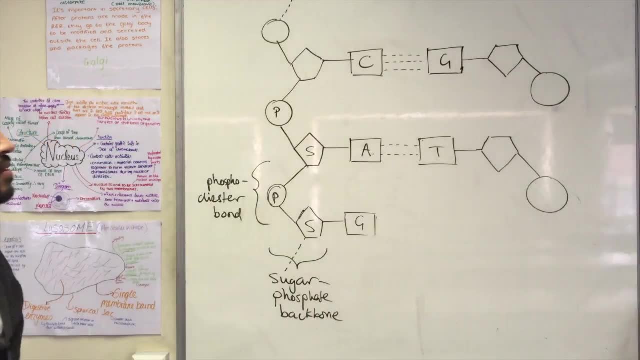 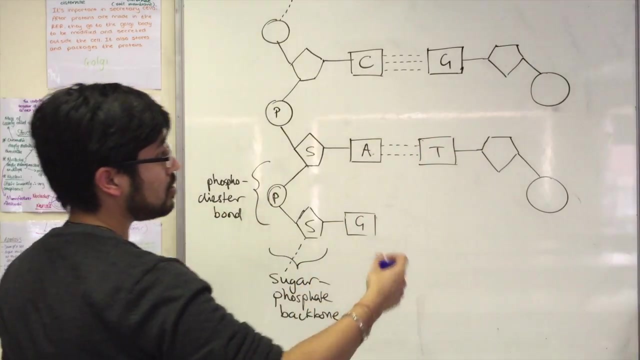 make two cells from one. Maybe that might have been useful to a very primitive cell a long time ago. Anyway, back to this. So you've got the nucleotides lining up and you've got a G here. so if we had a C nucleotide floating around, 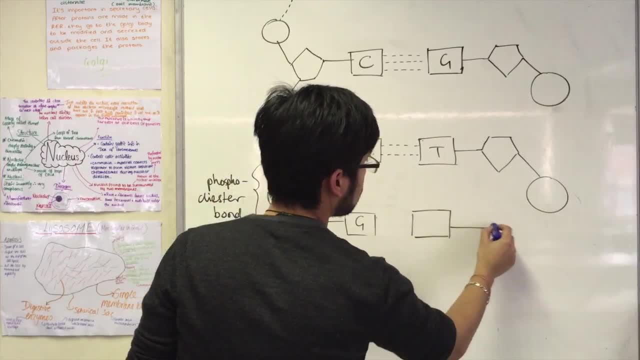 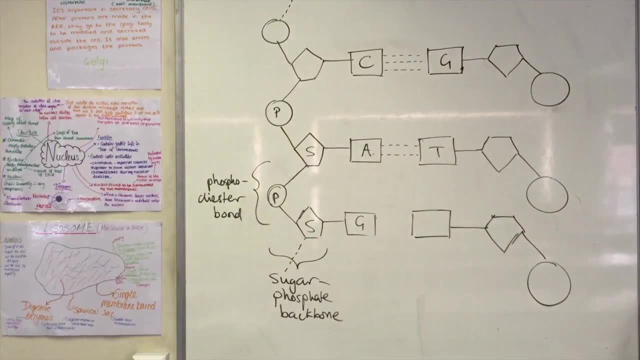 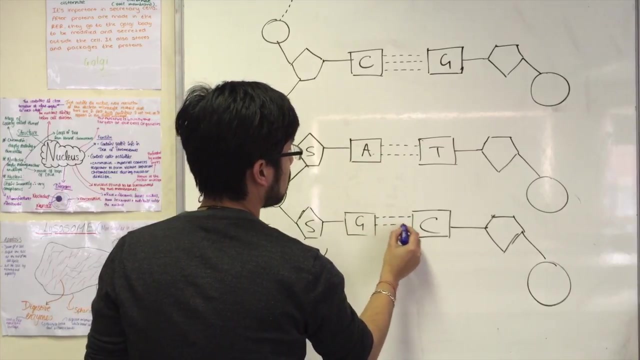 it would line up also Okay, Remembering that the bases have to be in the opposite- Sorry, the nucleotides have to be in the opposite orientation for that to happen, Okay. So when that happens, just like that, they'll form three hydrogen bonds. 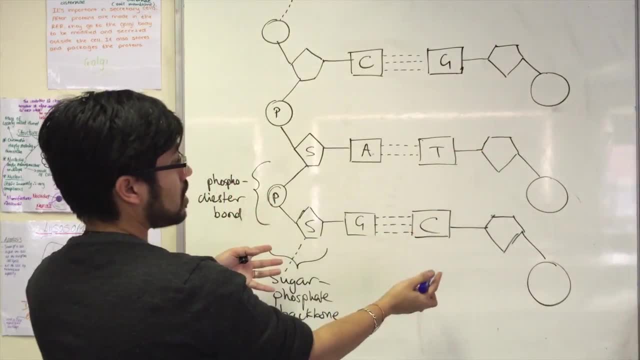 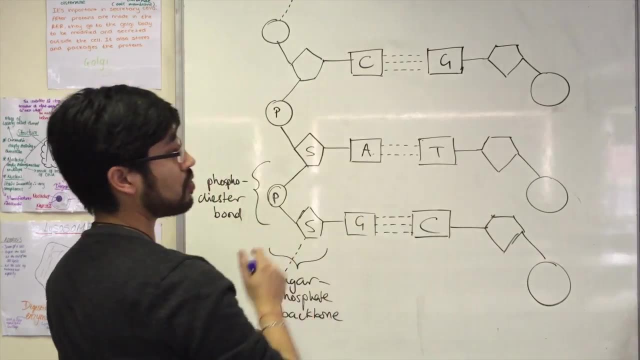 Okay, So you've got the nucleotides lining up because of the complementary base pairing which occurs because of the hydrogen bonding. Okay, This is important, And once you've got the nucleotides lined up, it would just take an enzyme. 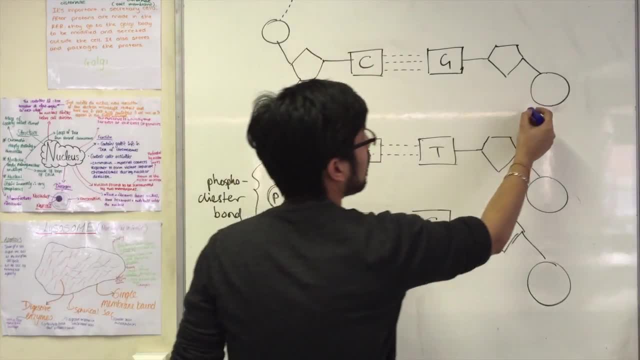 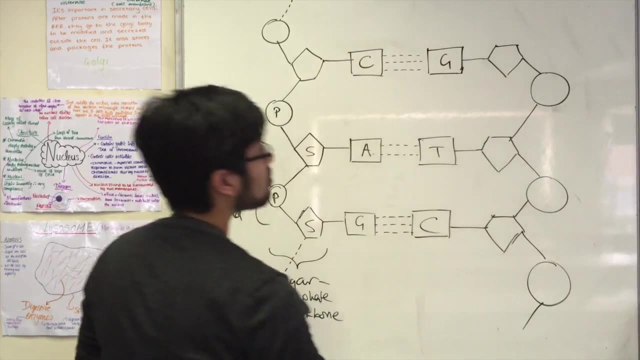 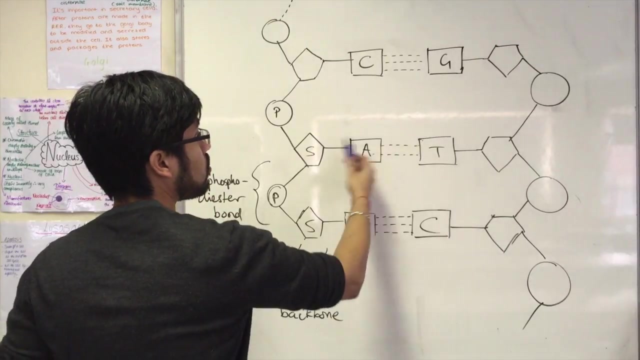 to be kind of following them, as they do that and form a phospho: an ester bond there, an ester bond there, and an ester bond there, and so on, until suddenly you had two strands with complementary base pairing. 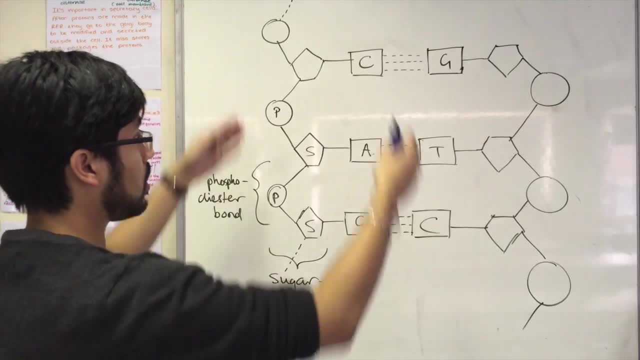 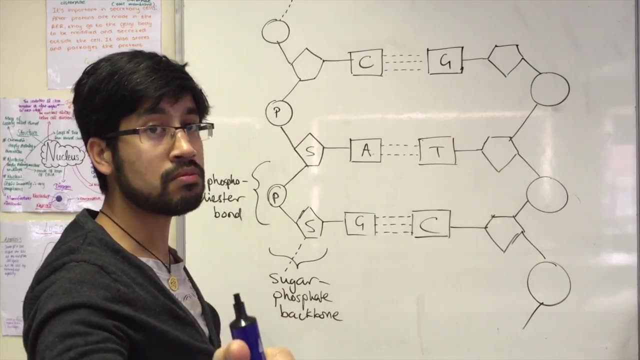 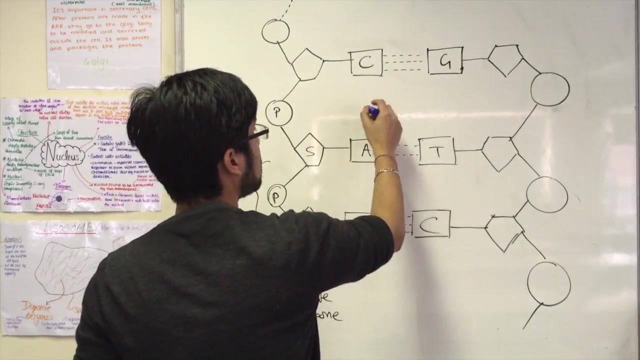 hydrogen bonding holding those two strands together and you have two strands of DNA. Is it a double helix yet? No, It's a double helix when these two strands start coiling, because these nitrogenous bases happen to be very hydrophobic. 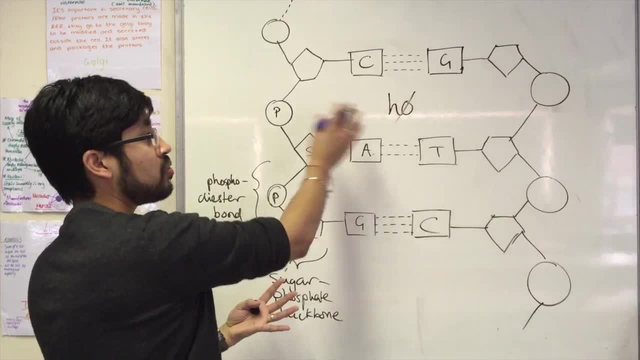 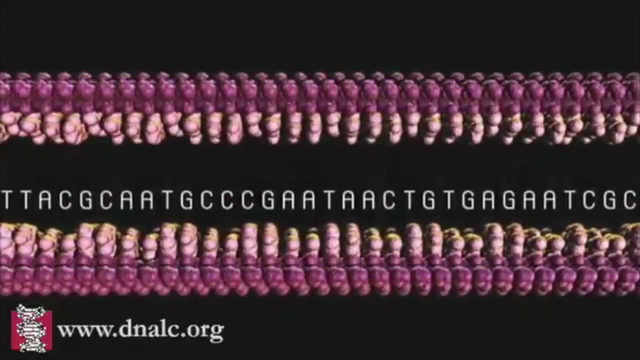 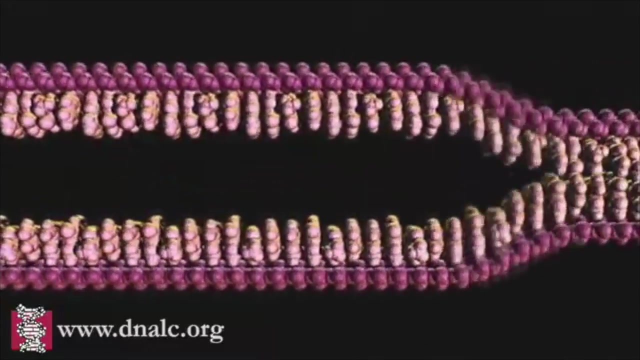 Okay, Two strands of DNA like this are exposed to the watery environment of the cell, Okay, But what happens is, because of the coiling, the bases are then shielded from the water. Okay, So the two strands coil up like this: 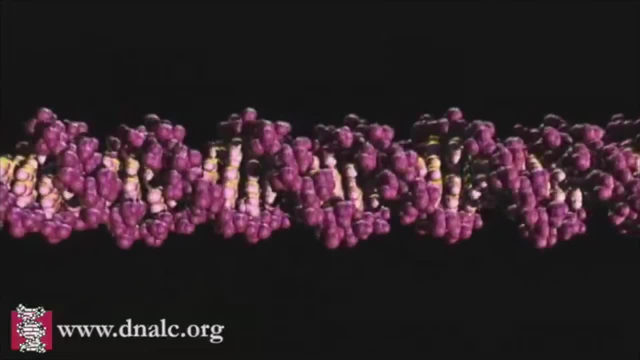 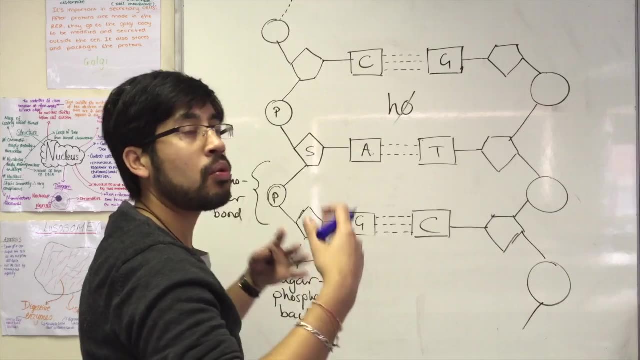 Bases are in the center of that coil away from the water. Okay, Similar to how the hydrophobic amino acids in a protein will be in the core of the protein, away from the surface. Okay, Right, So if this structure then coils, 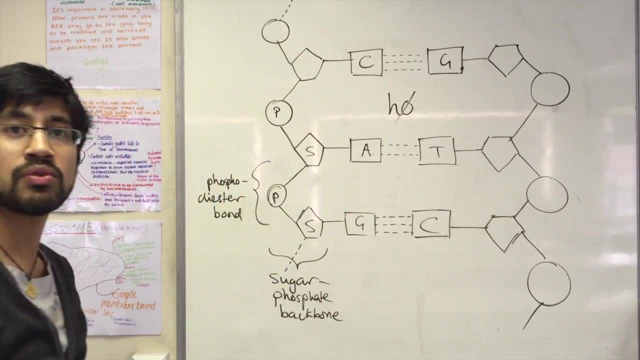 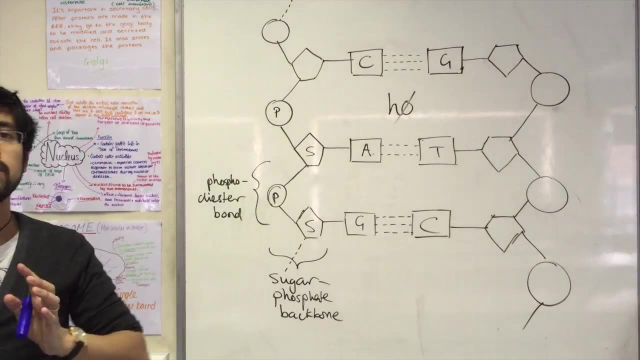 then we get the DNA double helix, But this is, you know, the essential structure of DNA. Okay, How is it? How is it adapted? well, not adapted? or how is it well-suited to perform its function? Okay,